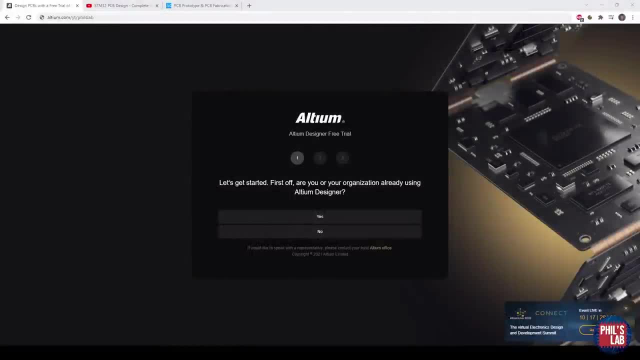 Thank you very much to Altium for sponsoring this video. If you'd like to give Altium Designer a try for yourself, they're offering a free trial if you go to altiumcom. forward slash YT, forward slash PhilzLab. There's a few Altium videos on my channel. 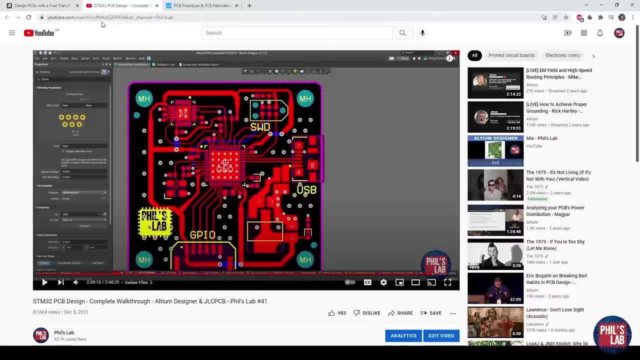 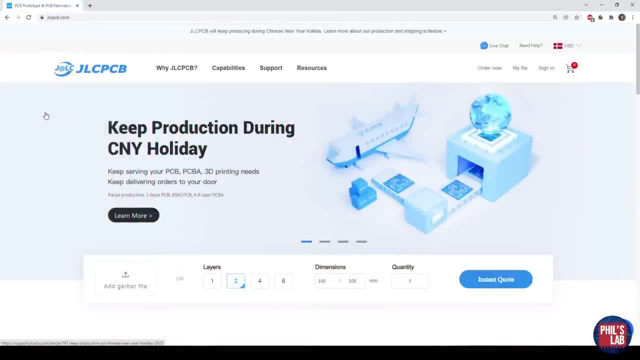 as well as KiCad. If you'd like a complete walkthrough of Altium, for example for creating an STM32 based PCB, I'll leave a link in the description and you can check that out for yourself. Thank you also very much to JLCPCB for sponsoring this video. I actually had 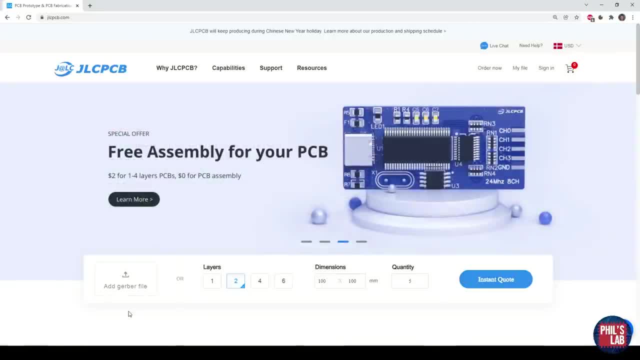 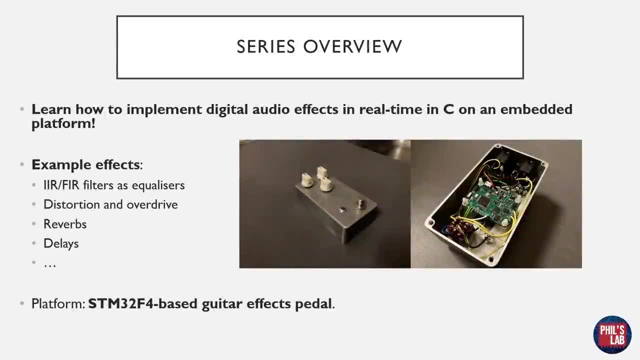 the Mixed Signal Guitar Processing Effects Board produced and assembled by JLCPCB. I'd like to make this series because I have a huge interest in electronics and audio, as well as digital signal processing, So I'd like to show you my way of how I implement. digital audio effects in real time. So let's get started. In this series, I'd like to explore several effects, starting with IRR filters, FIR filters, for example, for equalization, to start with, and then I'd like to explore some of the effects. 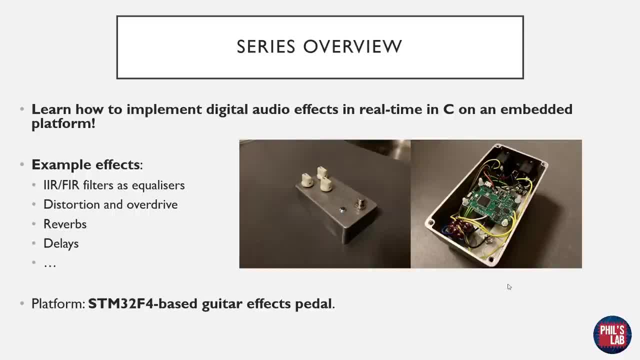 in real time using the C programming language on an embedded platform, And the platform we'll be using is this one here. Essentially it's a guitar effects pedal, but inside I'm using my custom GDSP core, which is an STM32 F4 based signal processor with an audio codec. 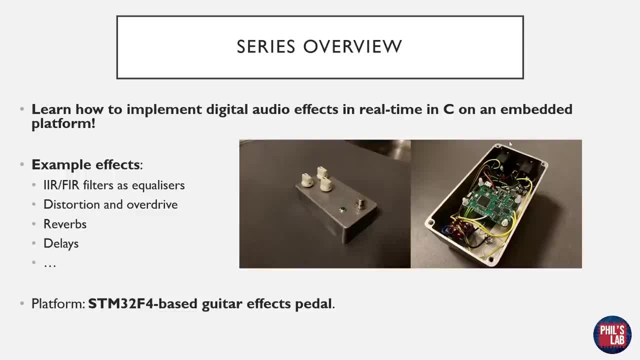 analog front end and so forth. We have an audio input from a guitar and an amplifier output, various controls and a footswitch to turn the effect on and off In the series. I'd like to explore several effects, starting with IRR filters, FIR filters, for example. 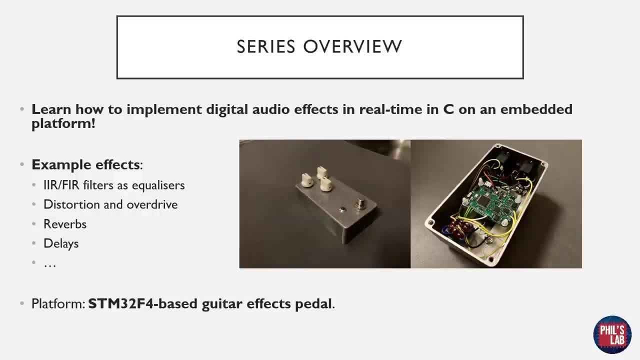 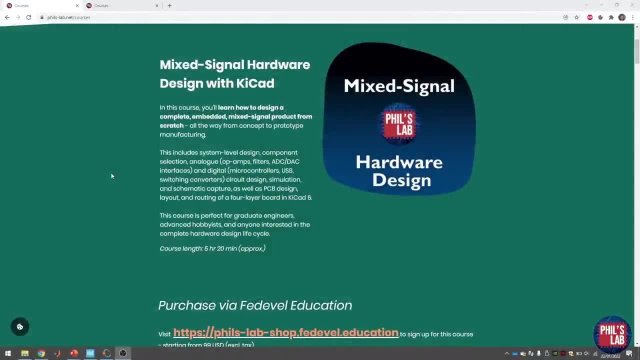 for equalization and we'll be using this STM32 F4 based guitar effects pedal. If you'd like to learn more about the Mixed Signal Hardware Design- and this is a board I also designed in KiCad- I've recently released a course on the Fedavell Education platform. 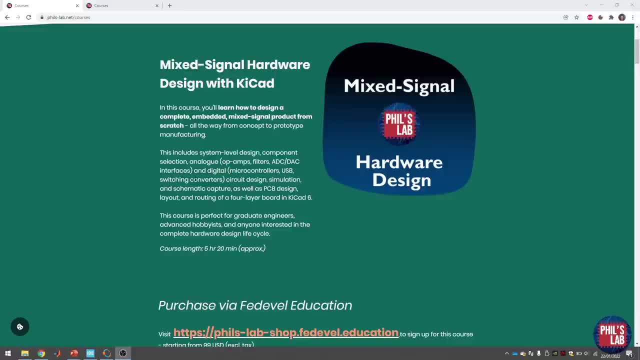 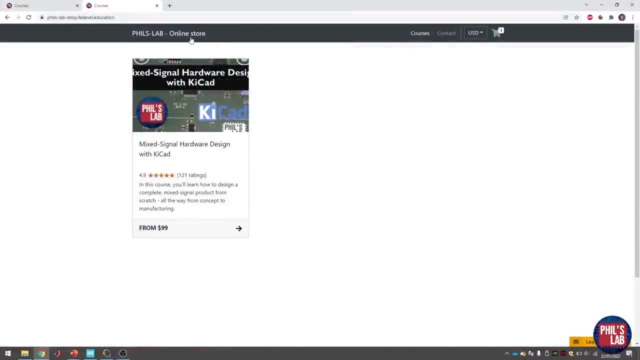 with Mixed Signal Hardware Design at its focus, where you'll learn to design pretty much a system like this, all the way from part selection and system requirements to getting the board manufactured. You can purchase the course via Fedavell Education and I'll leave links. 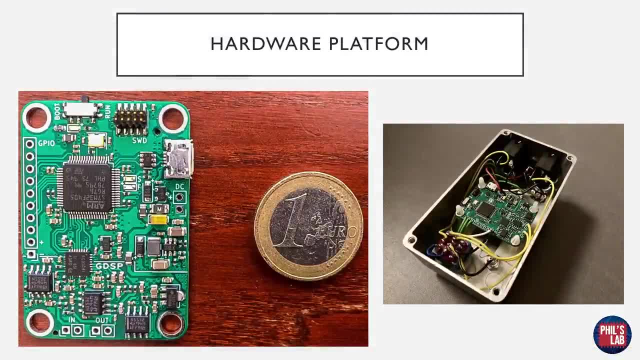 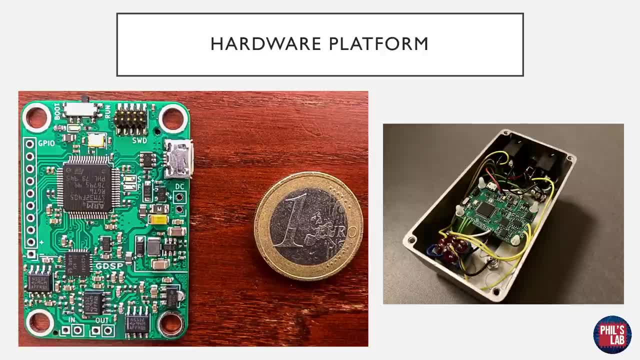 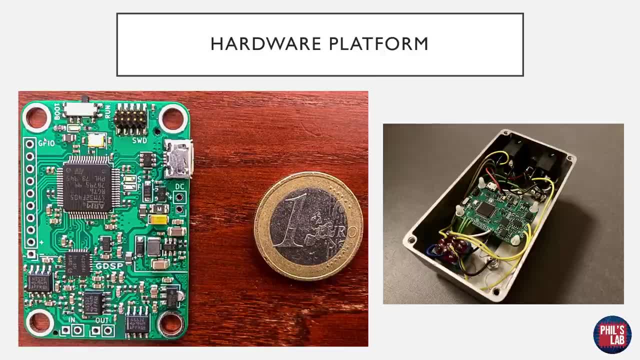 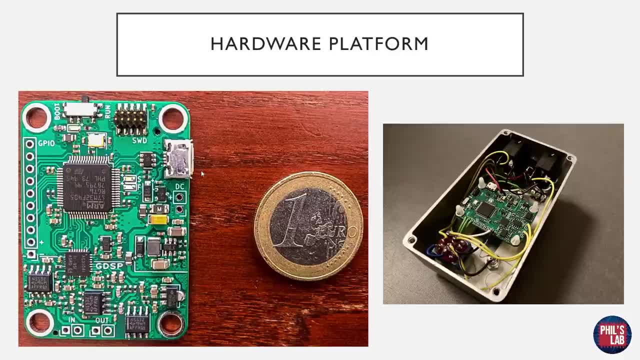 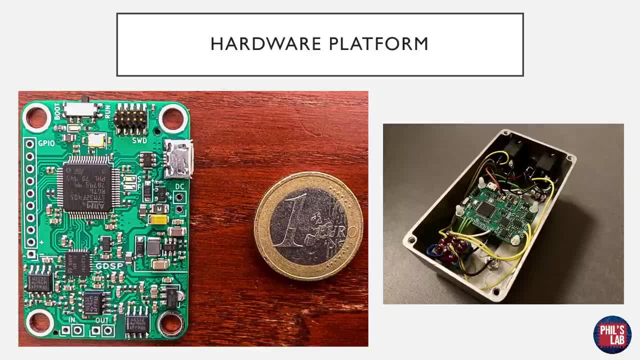 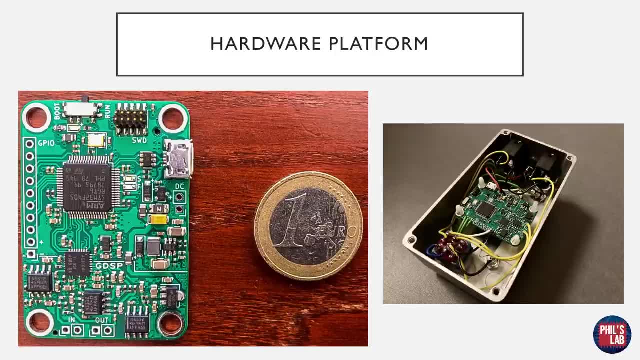 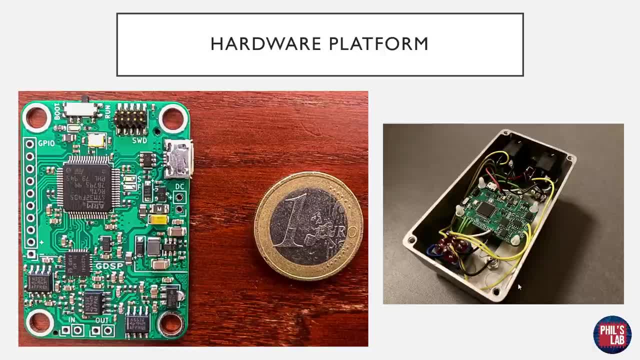 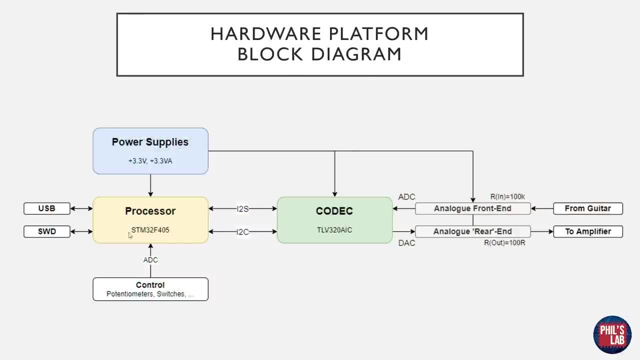 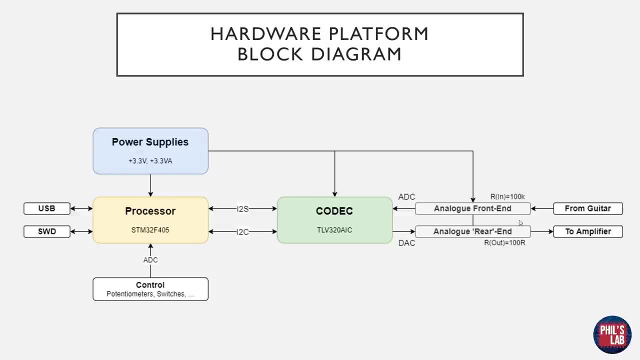 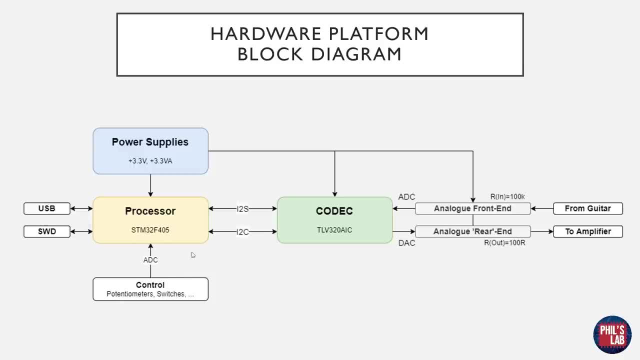 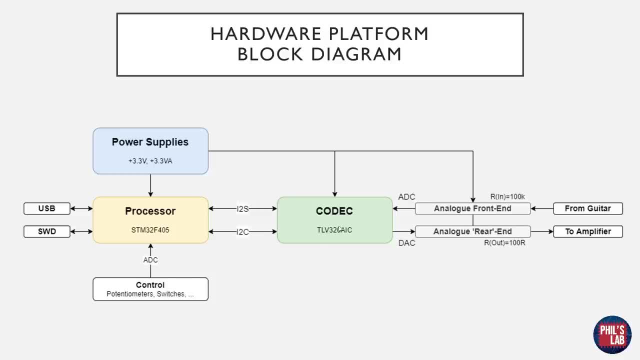 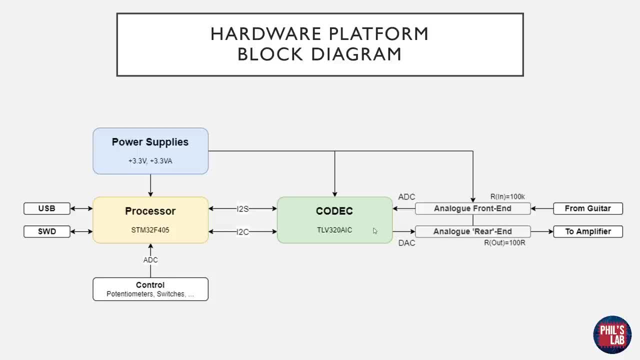 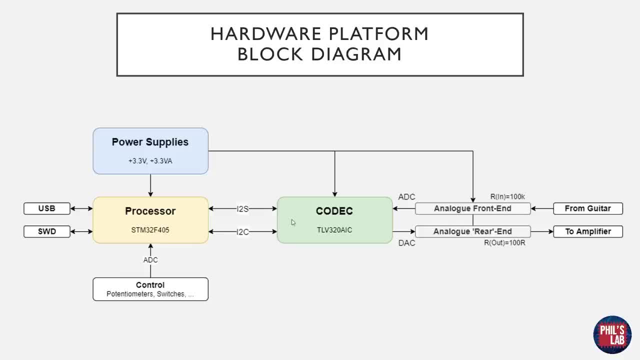 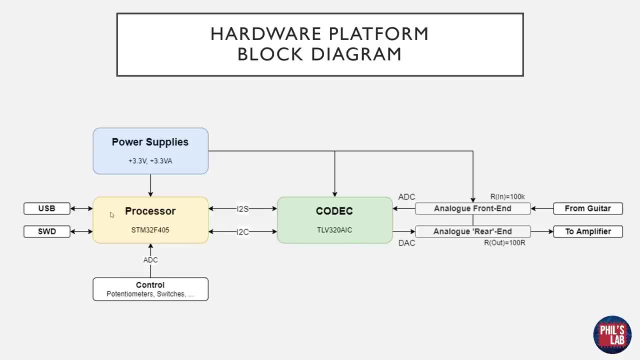 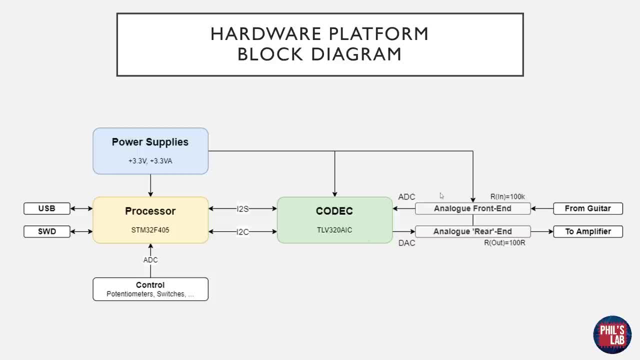 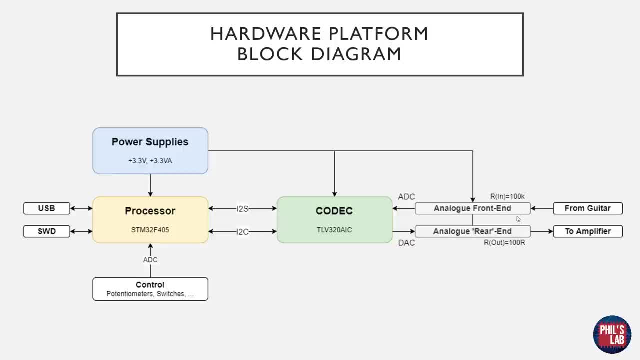 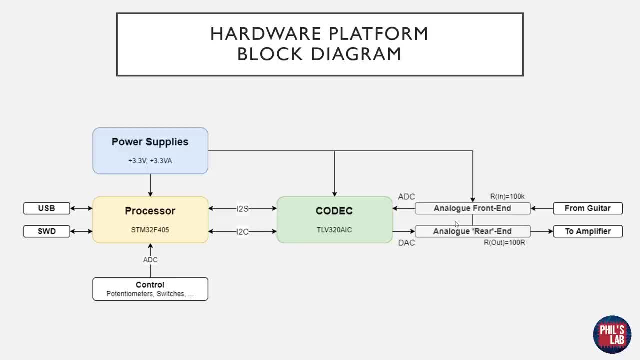 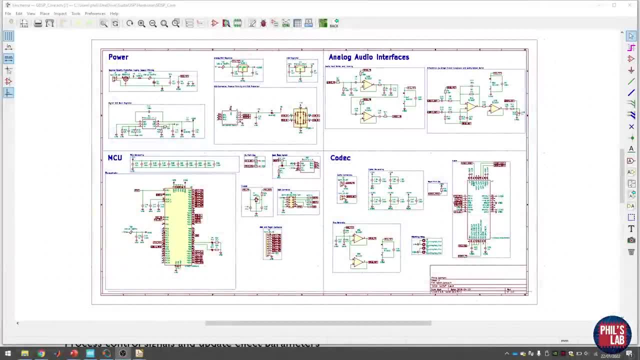 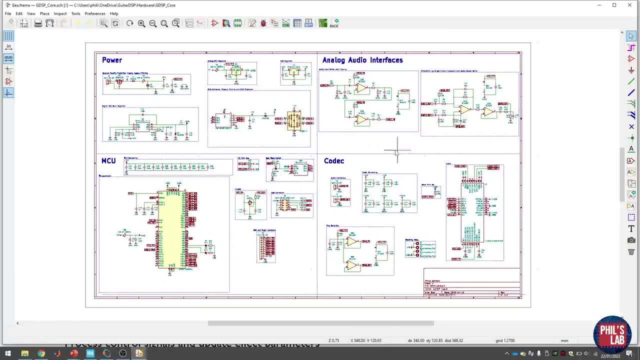 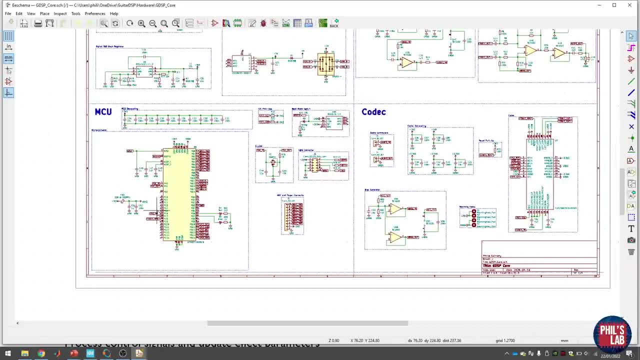 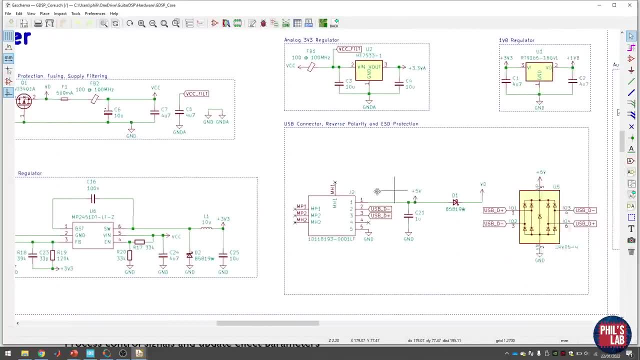 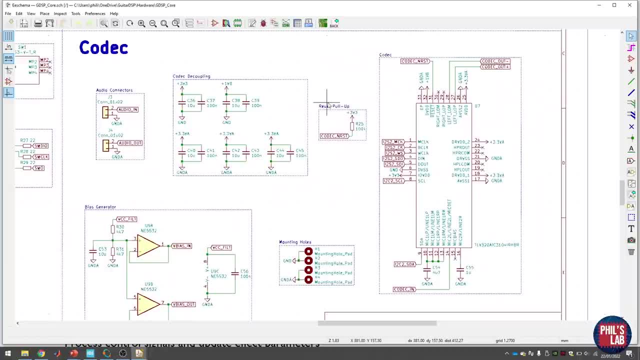 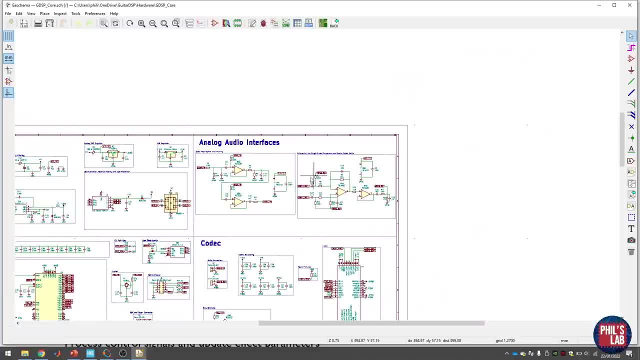 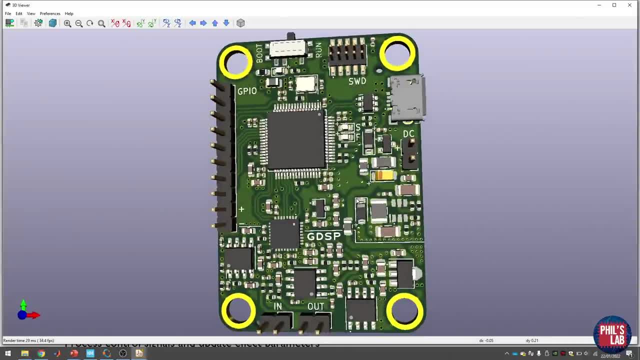 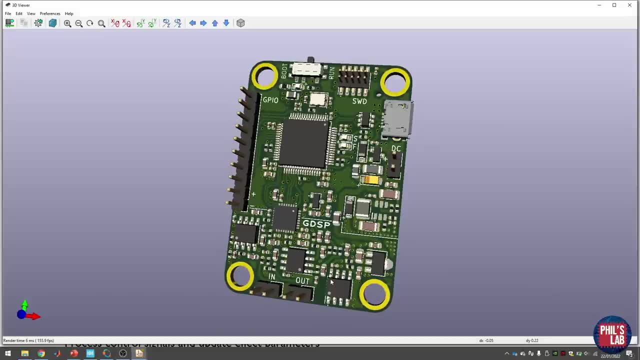 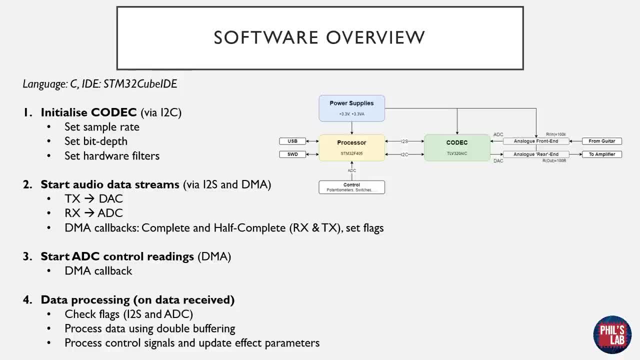 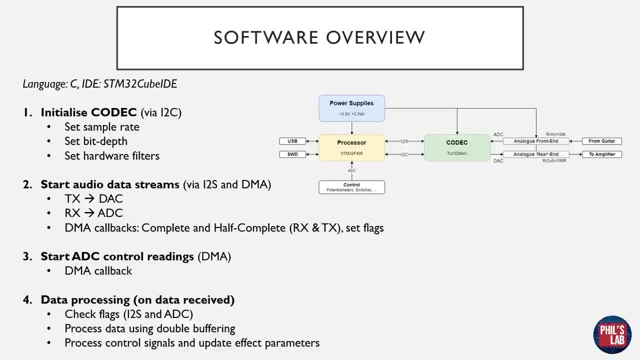 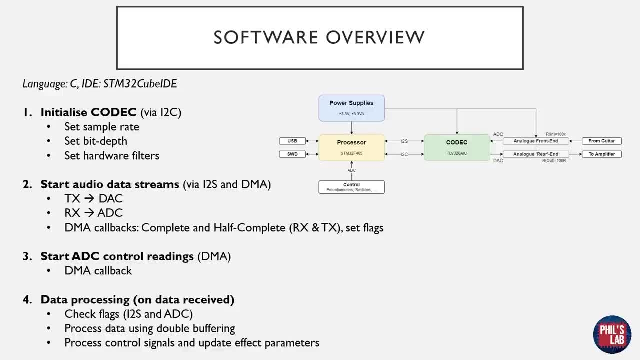 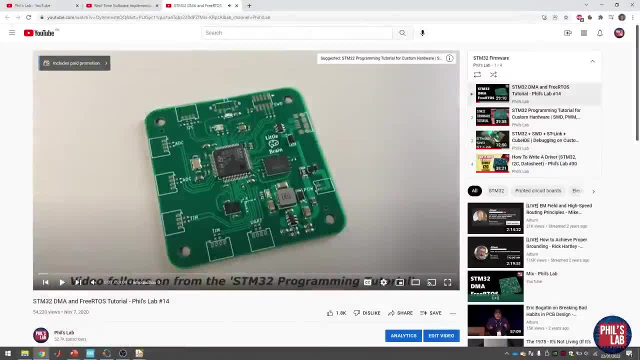 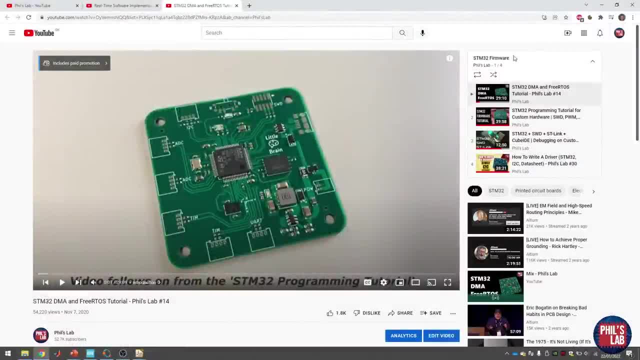 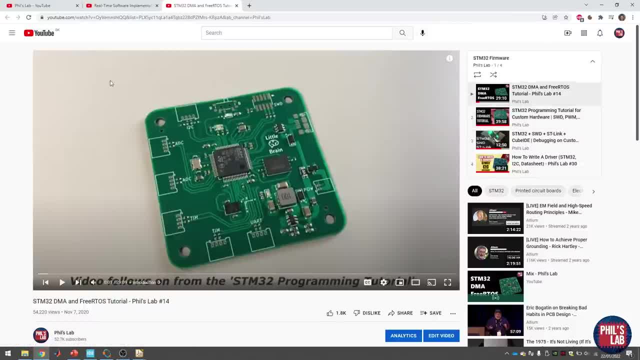 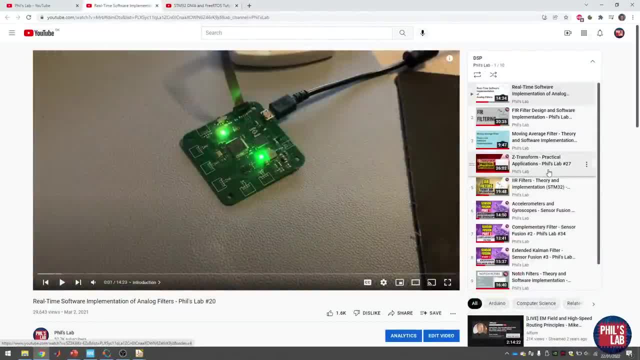 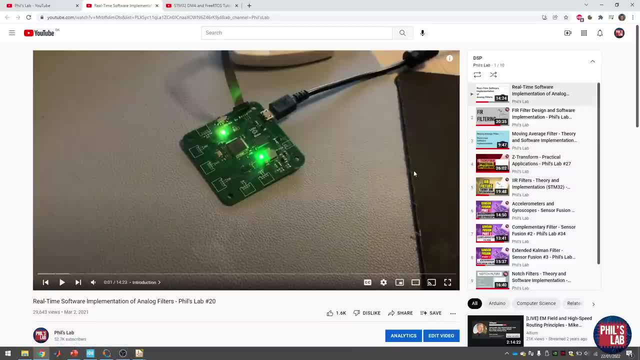 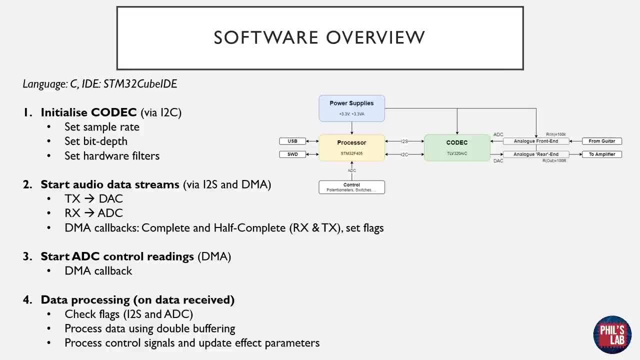 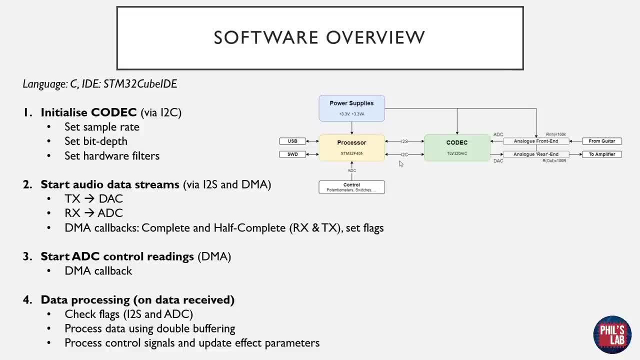 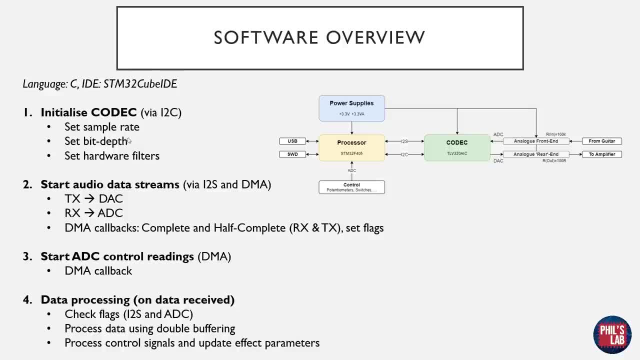 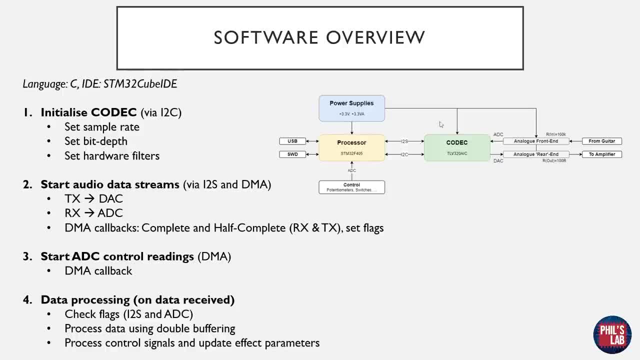 Here's an up close review of the course. Here's an up close review of the course. Here's an up close review of the course. might have some anti-aliasing filters or its own digital signal processing which you can enable via I2C. Secondly, we need to start the audio data streams. 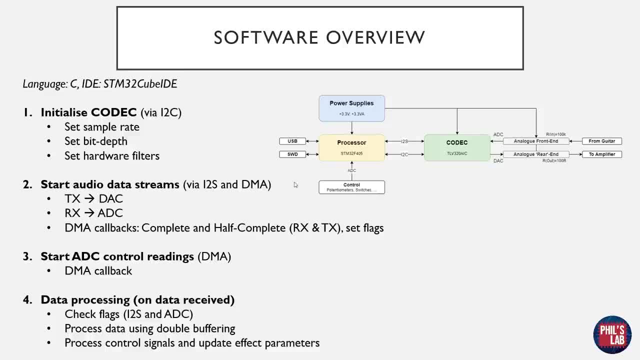 and this is done via I2S, which is very similar to SPI, and I'm also using direct memory access, which is DMA, and this really helps offload the CPU. Essentially, what I can do is use DMA to stream data in the background while the CPU is processing and applying our algorithms to our audio signals. So our 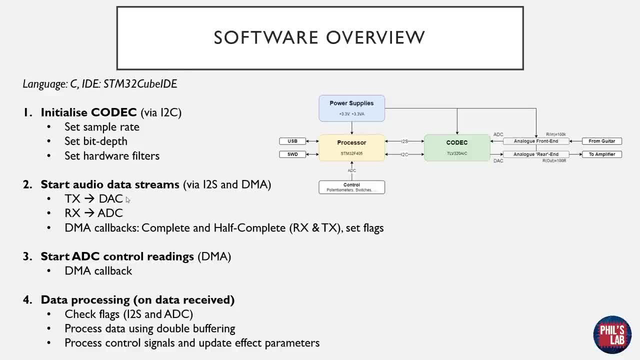 transmit stream via I2S and DMA will be to the DAC, so our output and our received stream will be gathering data from the codex ADC's. Nicely, STM32, and the processor we're using has DMA callbacks. We can let this DMA gather. 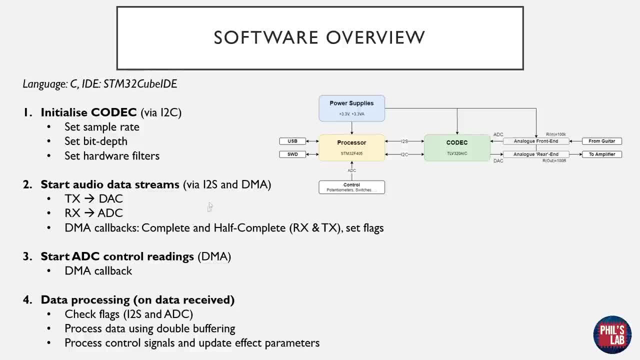 data and send data to the background, and once this has been completed, we will get some callbacks and then you're telling us: okay, it's done now and you can do some processing, and we get that for complete and half complete, so RX and TX, and then we can just set flags and we can read the flag somewhere else and 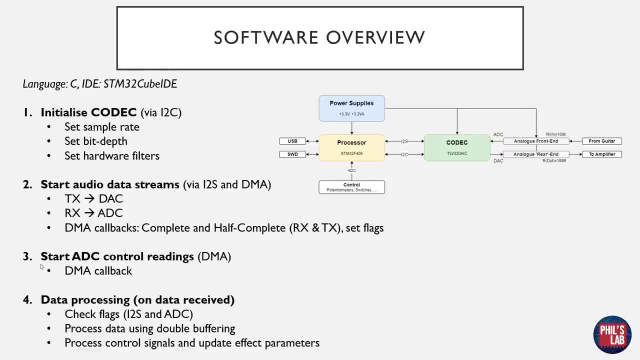 then process our data. So after we started the audio streams, we need to start ADC control readings, and the ADC in this case is from the processor itself, so these aren't suitable for audio, but they're suitable for reading, for example, control signals from potentiometers reading the voltage across a resistor, switches and so on. and 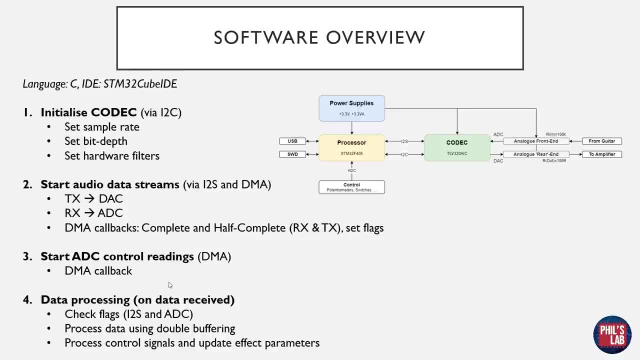 again, I'm doing this via DMA to offload the processor so we can focus entirely on processing our audio data. Again, we have a DMA callback that allows us to then process the ADC readings coming from these control signals. Now, these control signals we will use to, for example, change: 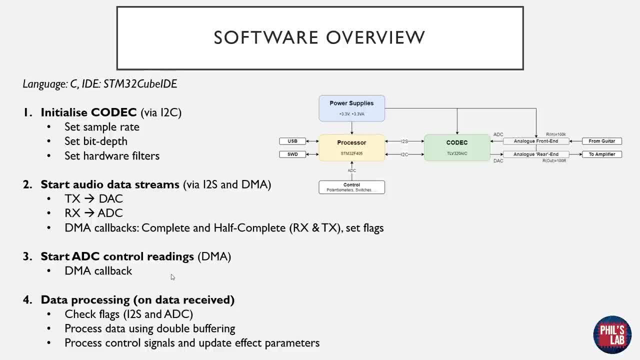 volumes. we can change filter parameters on the fly, for example, changing cutoff frequency, changing a Q factor, changing the reverb delay times and so on. so this is incredibly useful to have on a system. So once we've gathered our control signals and our data, we actually need to process that data, and to me, that is the 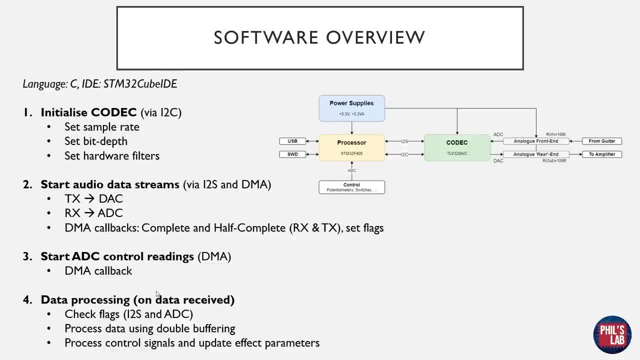 most interesting part and what this series will be focusing on. So once you have data received by these callbacks and flags, we need to check the flags and it's the I2S and ADC streams. we will process the data using what is known as double buffer. we'll look at briefly what that is in a second. then we need to process the control signals to get the data. 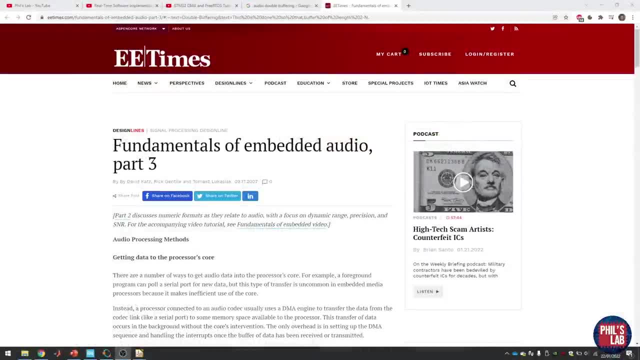 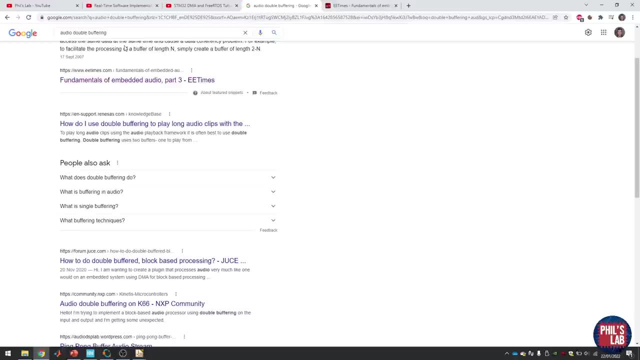 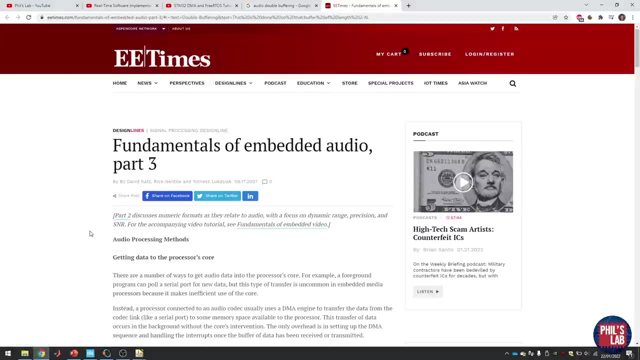 change our effect parameters and that's pretty much it. I briefly mentioned double buffering and if you do a simple Google search of what double buffering is, you can see it exists in graphics, but also in audio or any type of heavy processing. For example, this page on EE times gives a nice description of fundamentals of 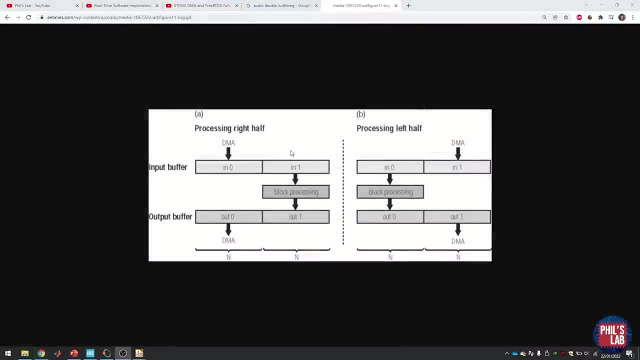 embedded audio and also on double buffering. So essentially for our input buffer, for example, we are using the DMA stream to fill that in from the ADC data into one half of this buffer. the other half of this buffer is being used to our processing of our audio signals and then fed to the output buffer Once we are. 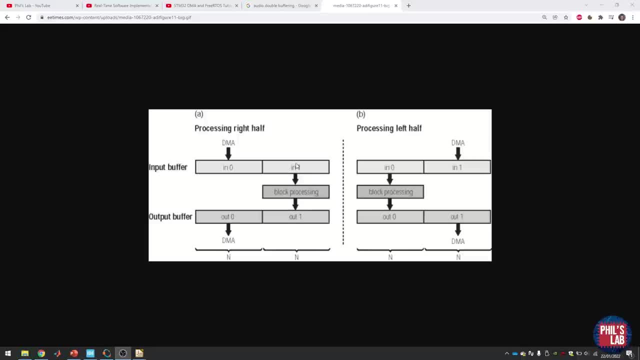 done with processing. the DMA stream will then fill up the other side of the buffer, which has now been used already, and then flip-flop between them. so every time we're reading in we're not using that part of the buffer to actually process. So always switching and making sure we're being very efficient with our 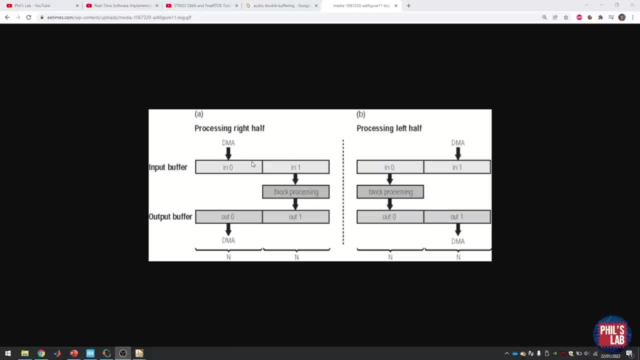 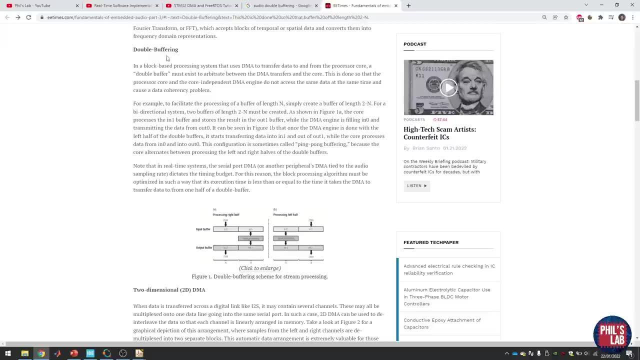 processing and also filling our data and retrieving our data. This works both ways for the TX and RX streams. So this was a very vague description and I really recommend that you read this up both on the EE times website and also just on Google, and I will leave relevant links in the 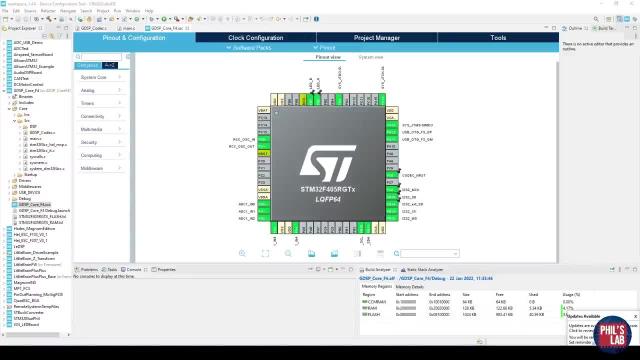 description below. Here we are now in STM32 CubeID and I briefly like to go through with you what I've already written for the firmware, and then we'll move on to actually implementing some filters and seeing the results and analyzing the results. The first thing I always do is take over the pin out from 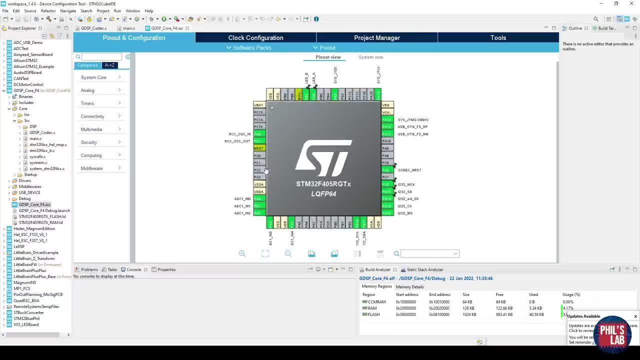 my key card or from my hardware and put it into STM32 CubeID. So you see, I've selected various analog to digital converters which will read my potentiometer values. I have my I squared S signals over here which connect to my codec USB CRY debug, as well as some LEDs and some various other signals I squared C. 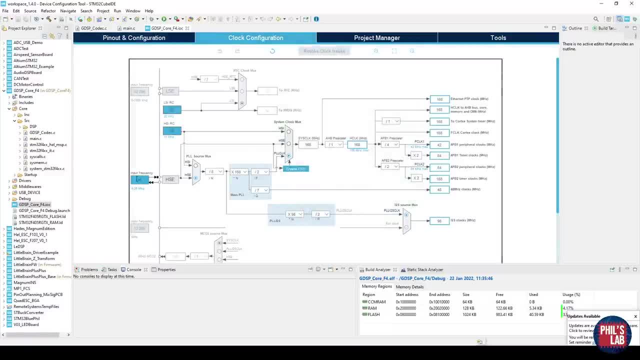 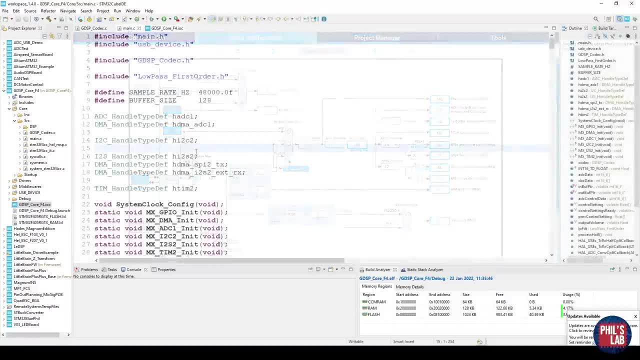 and my clock. Then I need to do my clock configuration. so I have an external oscillator at 16 megahertz and I'm running my MCU at 168 megahertz, which is the maximum it can do Now in my mainc file. this seems a bit complex, but 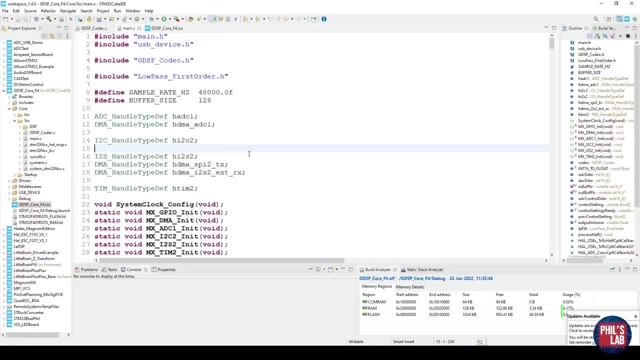 essentially, if you remember the presentation slides, we only have four steps. We need to initialize the codec, and I've written a driver, or very, very simple driver, in this codec file up here. We need to start our data streams and then we do the processing. So let's go. 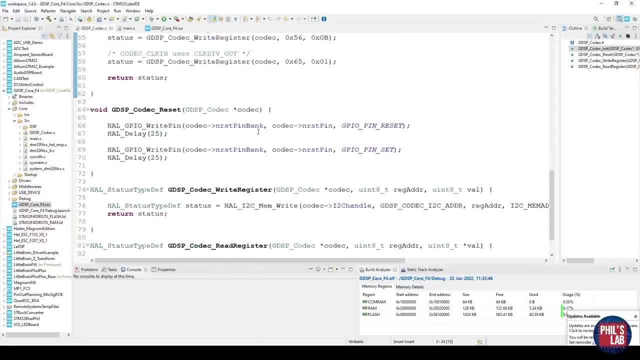 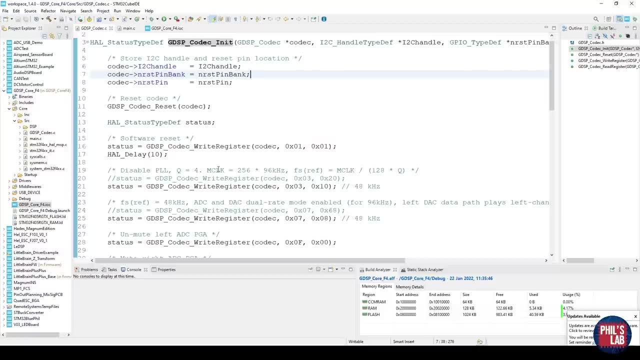 through that. So I've included my codec file. My codec driver is very shoddy and very simple just to get this up and running. So I'm doing software resets. I'm setting PLL values to make sure that I'm getting the right sample rate, So I'm 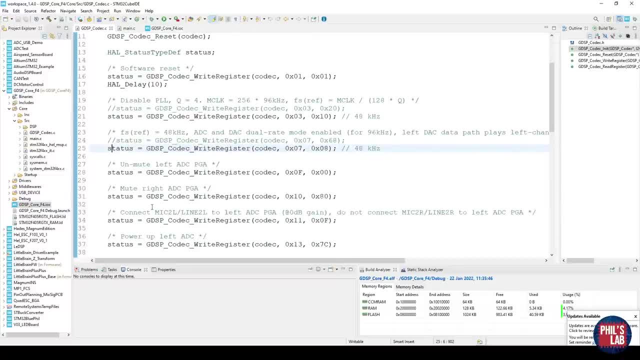 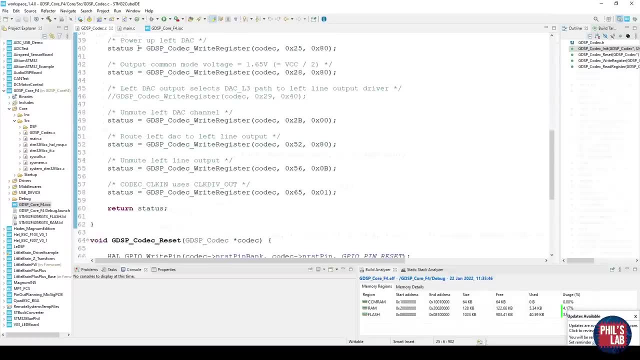 setting my sample rate to 48 kilohertz, and this will be important later for processing. I'm unmuting the various channels, powering up the codec and so forth, And all of this I've done via the help of the datasheet. So the first thing, 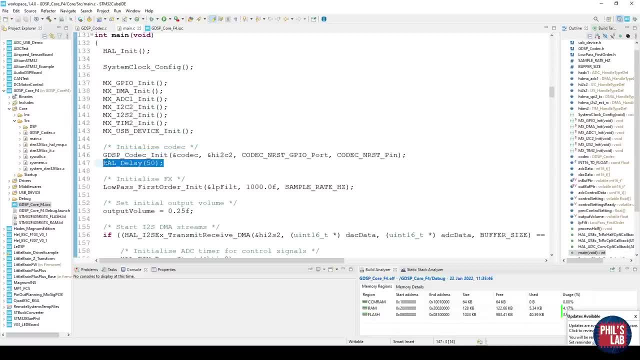 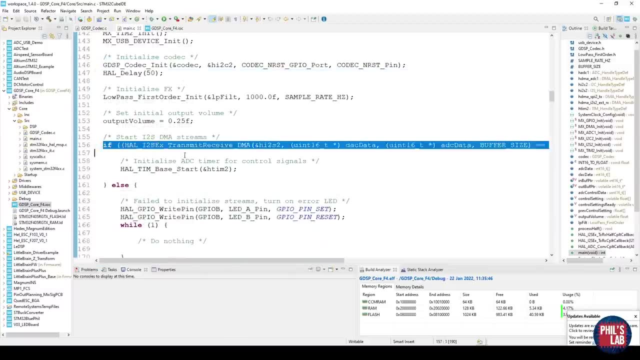 I initialized is. I initialized my codec and I wait a bit to let it settle. very loosely speaking, We'll come to this later. but then I initialize my effects, set my outer volume and then I start my data streams. So I use this here, which is: 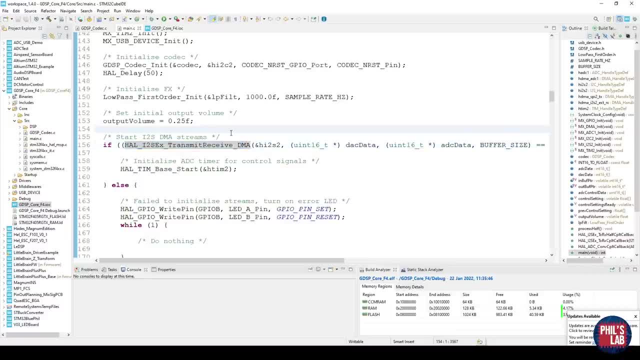 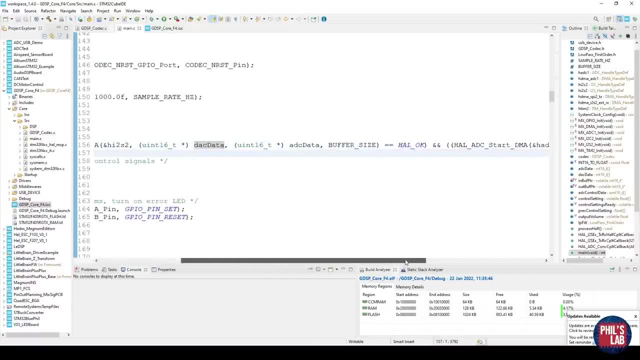 a transmit- receive command and I'm using the hardware abstraction layer provided by SM32, starting my DMA data stream and filling in my buffers for the DAC data and ADC data, And if this works out for both ADCs and for the codec, then I will. 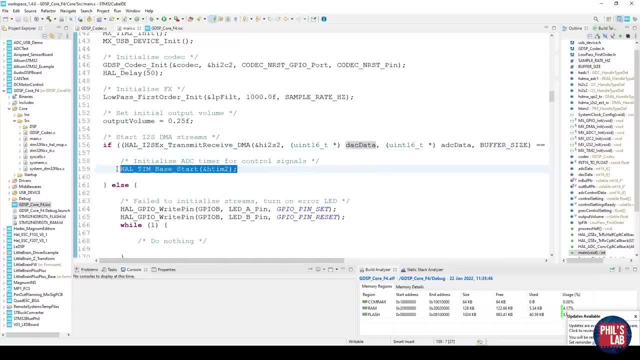 start my sampling rate timers and I'm using a timer to trigger the reads, for example, of my ADC at about a hundred Hertz or kilohertz. This timer for the ADC is for the control signals and the control signals don't have to be sampled that often because I, as a human, am changing. 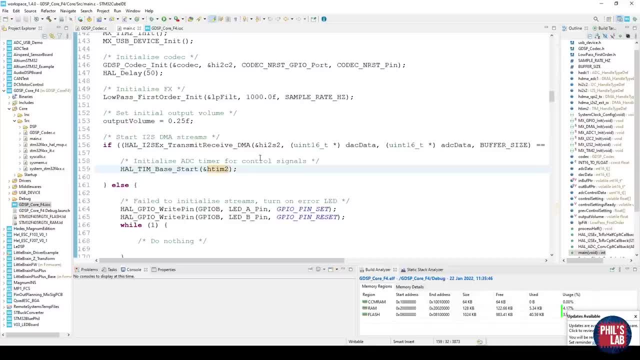 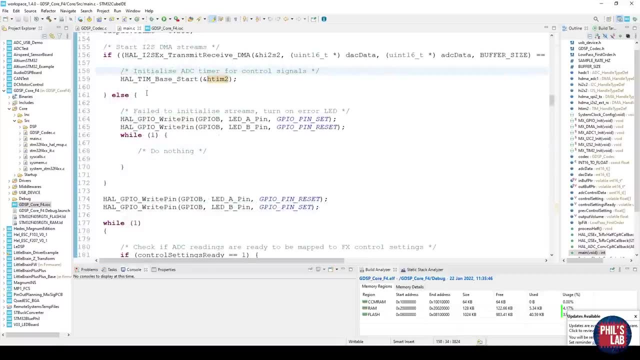 these and I'm changing them, you know, once in a while, So we don't have to sample the control signals, for example from the potentiometers or switches, too fast. So 100 times a second is more than enough. So once we are okay with starting, 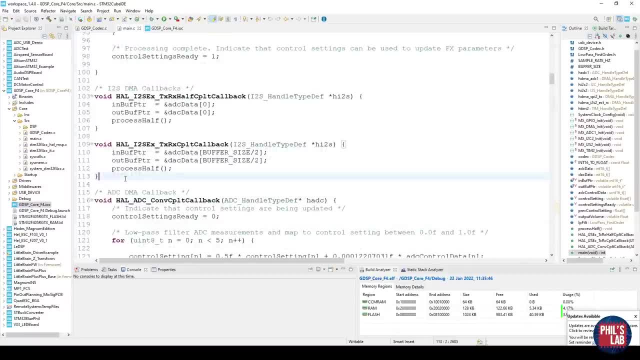 the data streams, we do our processing and our while loop. Before we can process, however, we need to do our double buffering. This happens in these I2S callbacks over here. I will leave a link to a video below in the description that will teach you more in double buffering also. 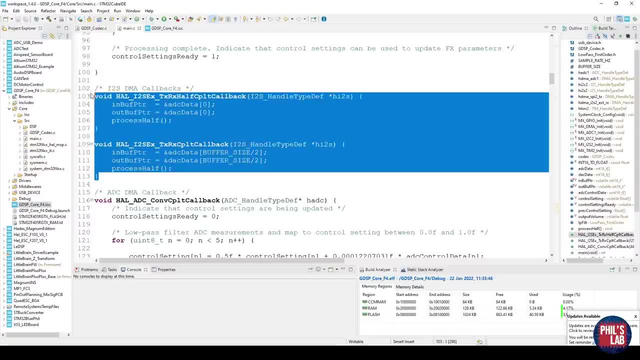 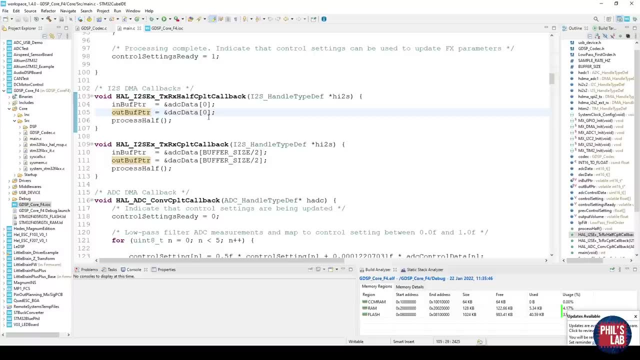 specifically to SM32. And this is the kind of structure one would have to implement. essentially, you're, rather than moving data, you're moving pointers around, depending on what if you're receiving, transmitting or processing For the ADC. we don't need to double buffer. this is the ADC of the control. 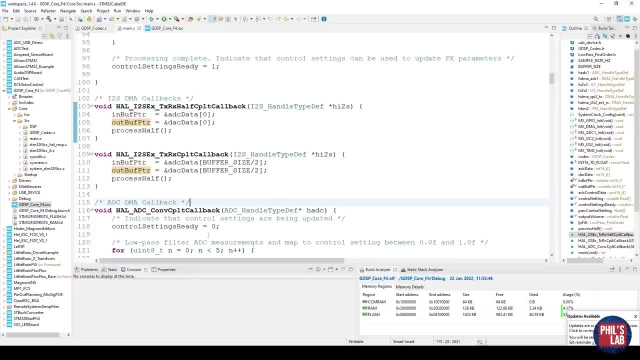 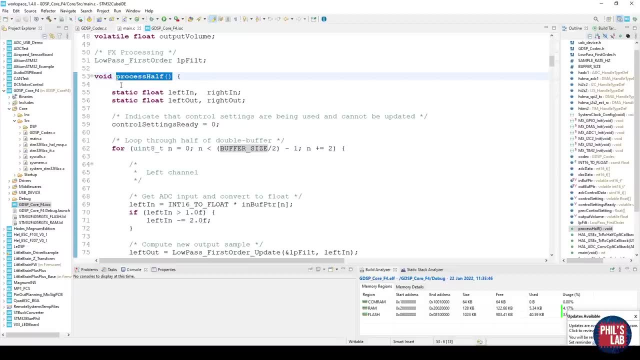 signals and essentially I'm just converting my raw ADC readings to control settings between 0 and 1.. Our main processing function is called process half because essentially we're just processing half of our buffer. Again, this is to do with the double buffering. We have left inputs with right inputs. 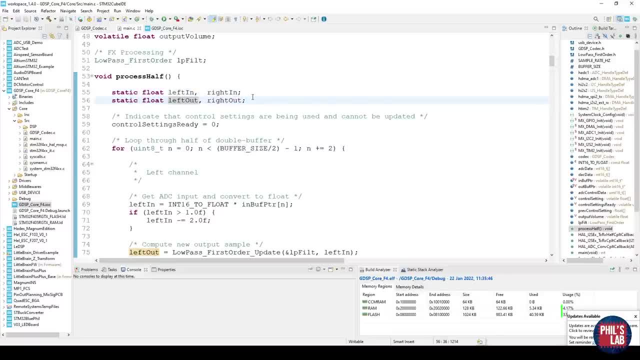 because it's stereo, and left outputs and right outputs. Now, because I'm using this in a guitar effects: pedal and guitar effects are typically mono. we would just be using the left input and the left output, And this process, half function, is our main processing function and where we 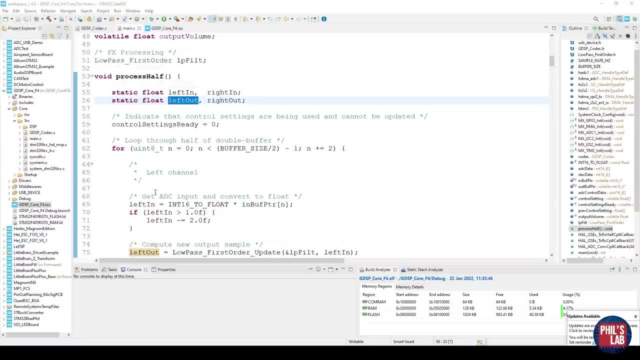 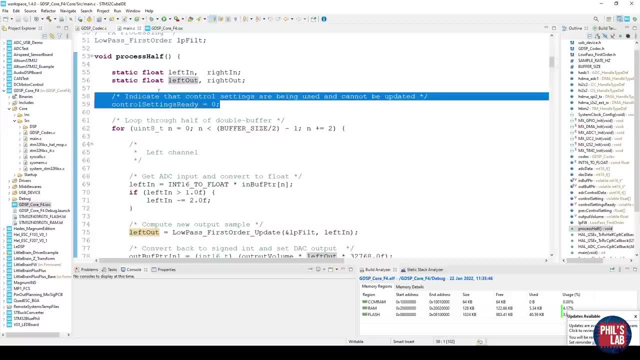 will be implementing our filters and our code, or at least calling them Very briefly. we make sure that during that time we are processing that the control signals do not change. so we indicate that with this flag to make sure we don't get any strange artifacts: that while we're processing maybe the control signals change and that will. 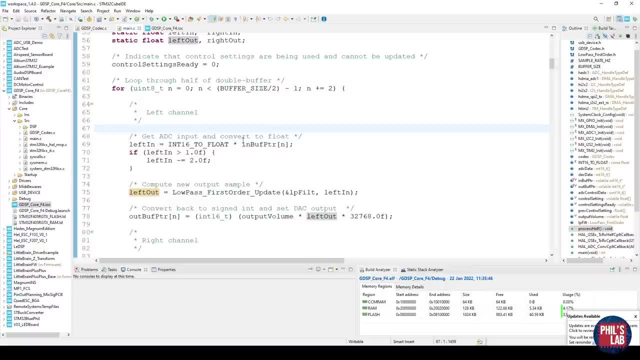 mess up our sound. So we loop through half of the buffer, starting with the left channel. we get our ADC input, that is the ADC from the codec, and convert that from an integer to a floating point value and then do some sort of scaling. and this depends on your codec and the way you're reading. 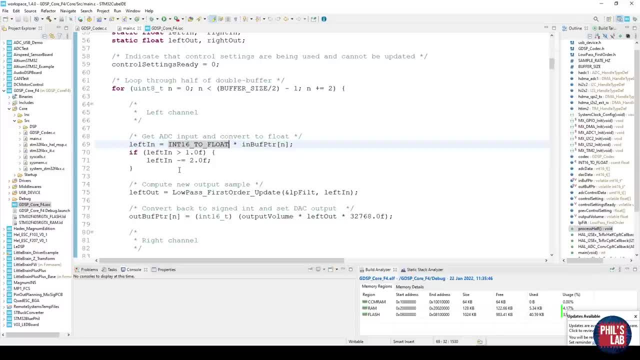 it in. I prefer working with floating points. it's less efficient, of course, but if we're just demonstrating various algorithms and we're not too concerned about speed because we have enough processing power, this is the way to do it. Work with floating points, it'll make your life so much. 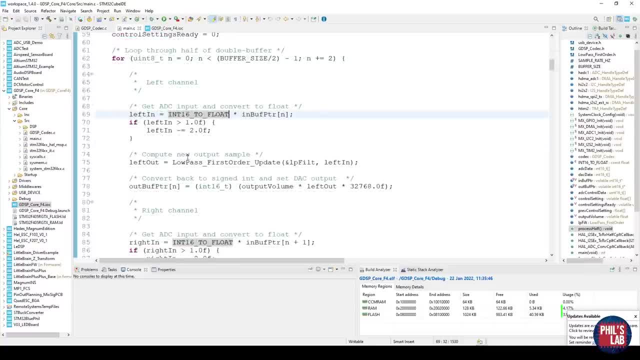 easier. Then we of course have to compute our new output sample- and we'll look at how to do that in a second- and then convert it back to a signed integer to set the DAC output in the buffer. We do the same thing for the right channel, and that's pretty much it. So what we need to do in 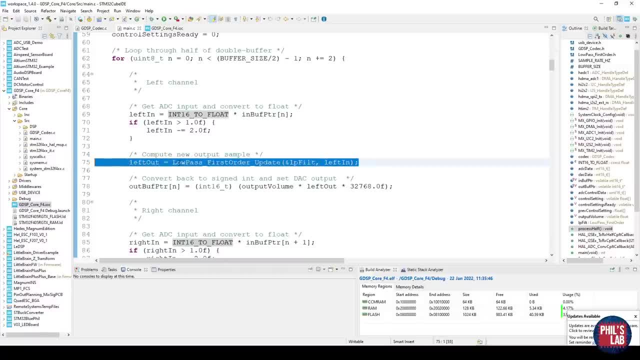 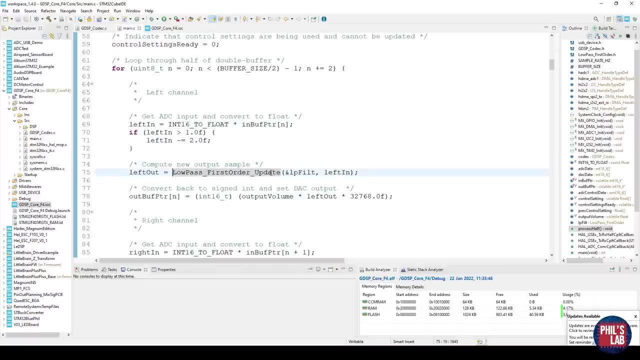 this series is compute, the output sample, and this will depend on if we're doing filtering, if we're doing reverbs, delays, distortion and so on. In this video I'd like to show you low and high pass filters. I understand this is a pretty vague explanation of this code, but it's basically to give you an 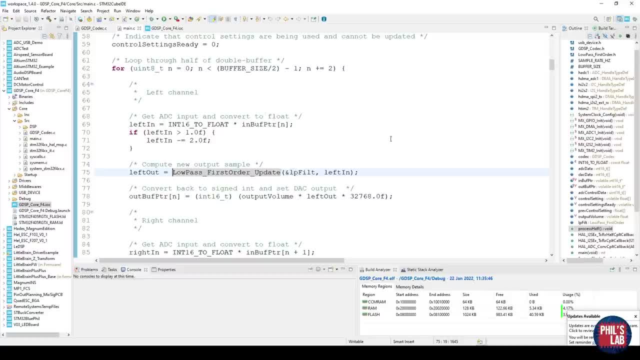 introduction and overview of what parts of the code you will need. so if you'd like to follow along, I will leave code in the github repository and I'll leave the link to that below. In this series, we are simply focused on actually then writing the audio algorithms rather than writing 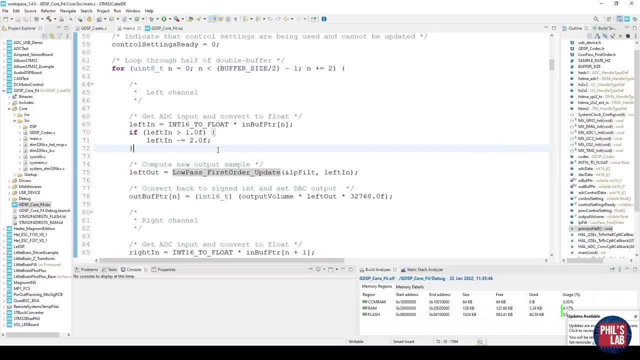 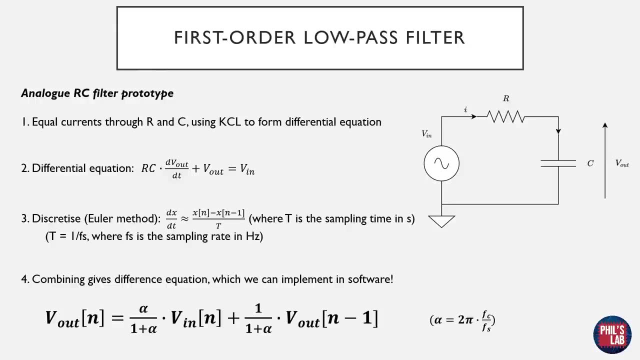 the drivers. so I'll give you this framework without much explanation, but if you have any questions, please leave them in the comments below. What we'll be implementing today are, first order, low pass and high pass filters. Now I have a video on my channel that goes in far greater detail of how to derive filter models from analog prototypes, but I will 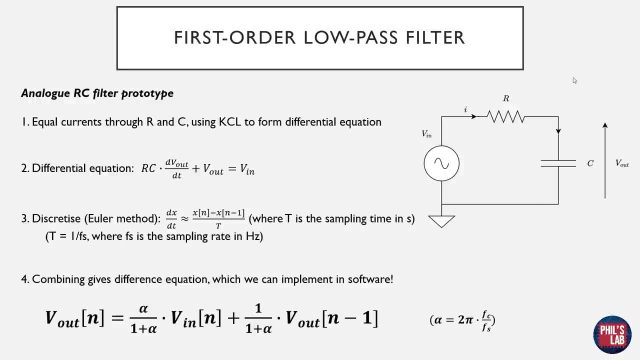 just run through the basics in this video. In essence, we'll be using this RC prototype filter, which is an analog filter, as a prototype, and then moving over and discretizing this to give us a difference equation that we can then implement in software. First thing we have to assume is that we 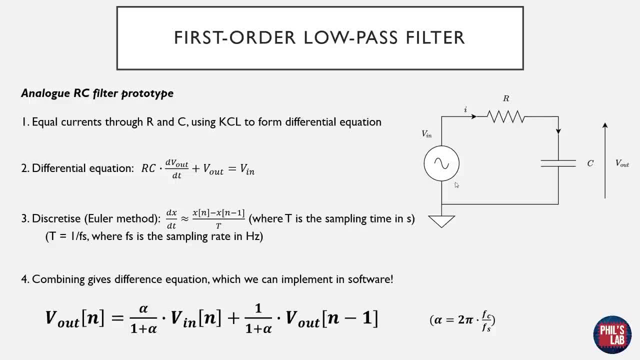 have equal currents through this resistor and this capacitor. We have a voltage source on the left, which is our input voltage. we pass this through our filter and we take the output across this capacitor over here. So again, assuming equal currents through this resistor and this capacitor. 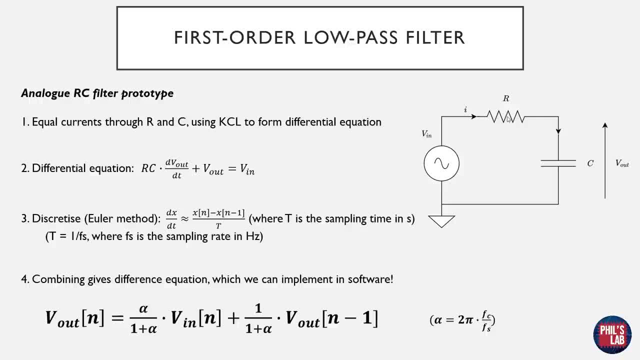 through the resistor and capacitor, we can use Kirchhoff's current law to form a differential equation. Differential equation then turns out to be this one over here. so RC times dv out by dt plus v out equals v in. This is, of course, is in the continuous time domain, and we want to go to the. 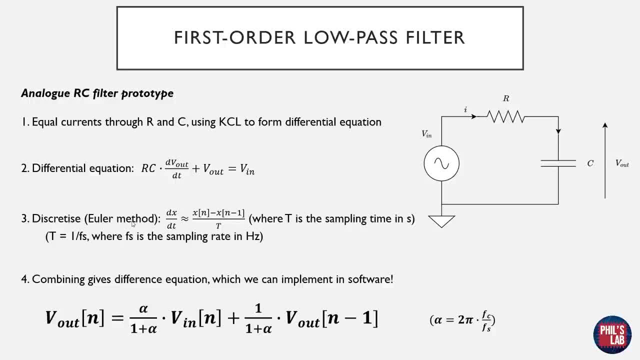 discrete time domain, so the digital sample domain. The way we do that, there are several methods. the easiest one is to discretize using the Euler method. Euler method says that we can approximate derivatives by a first order approximation, letting that dx by dt is approximately equal to the 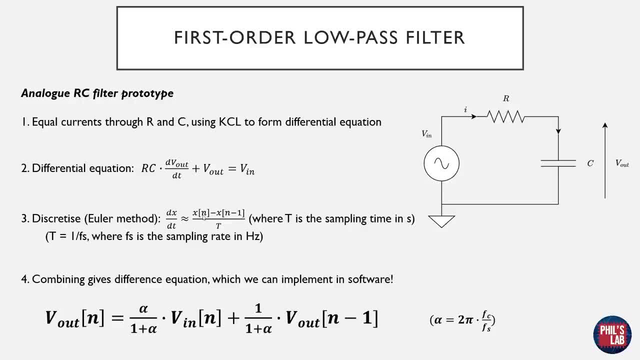 difference in size. So that's the first order approximation and the second order approximation is the second order approximation. So that's the first order approximation. So, for example, dx by dt is x at sample n minus x of the previous sample n minus 1 divided by t, and t is the sampling time. 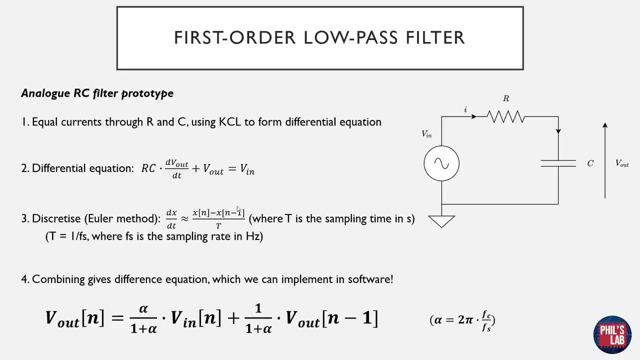 in seconds. So this is the discrete derivative. essentially, t is the sampling time in seconds and t is also 1 over fs and fs is the sampling rate in hertz. So what we then need to do is for dv out by dt. use this expression for dv d out by dt, plug that in and also make sure that v out. 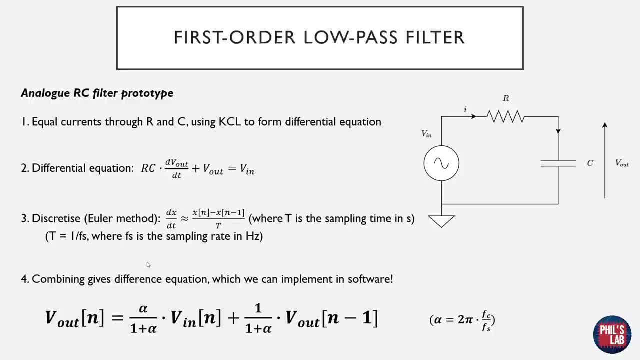 is then sampled and v in is sampled. So that's the first order approximation and the second order approximation is the first order approximation. So combining all of that information gives the difference equation which we can then straightforwardly implement in software. So we have v out sample n. so this is the latest sample. is this constant over here or this? 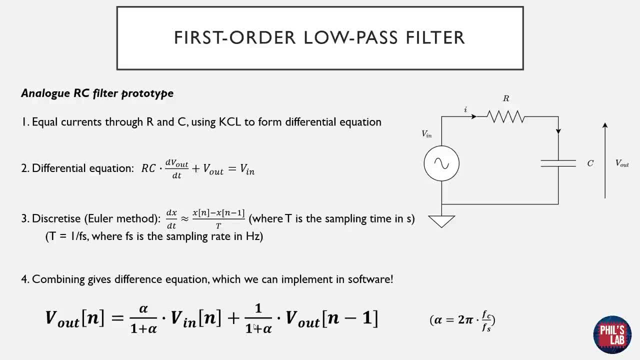 coefficient times the latest input sample plus a different coefficient times the previous output sample. Now I've written it in terms of alpha and alpha over one plus alpha and one over one plus alpha, because these are reoccurring terms and alpha actually is two pi times the cutoff frequency in. 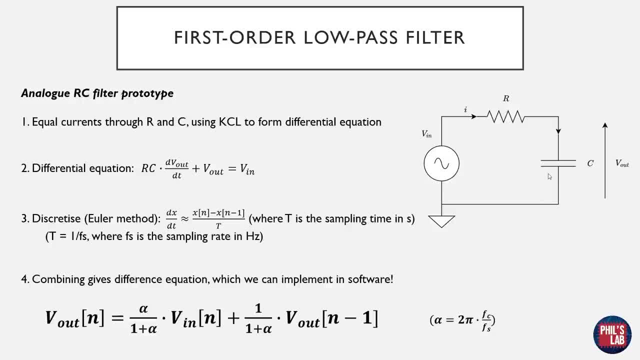 hertz divided by the sampling frequency. If you remember, for RC filters the cutoff or the minus 3d b point is defined if fc is 1 over 2 pi RC. So instead of using resistors and capacitance values, I'm just using a cutoff frequency, because you know it doesn't really make sense to that. 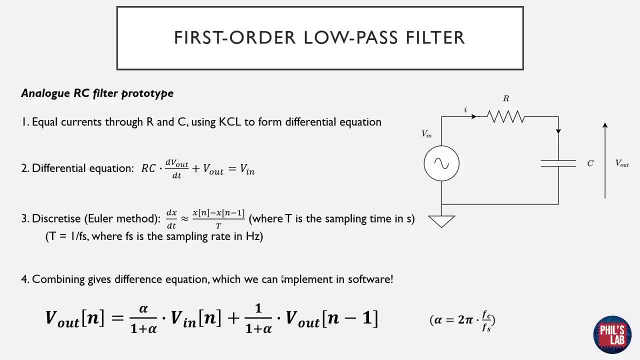 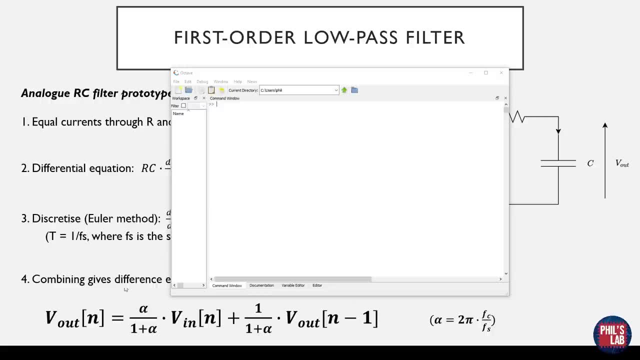 digital domain. So alpha is 2 pi fc over fs and we can use that and that gives us a first order low pass filter. I can use MATLAB or Octave, which is the free alternative, to plot the frequency response of my discretized filter. So let me do that now. What I need to enter is my sampling. 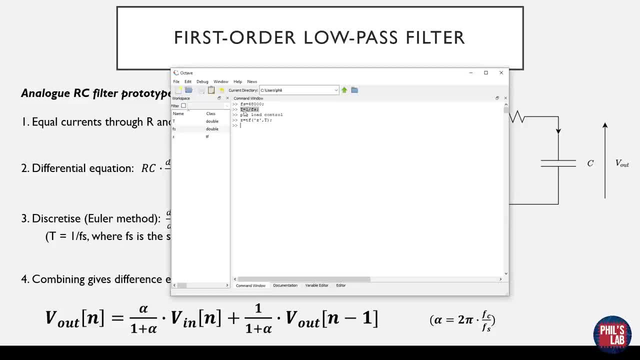 rate which is 48 kilohertz, then I can convert that to a sampling time or something like that Period which is 1 over sampling rate. I need to load a package called control because I want to work with a z transform. Now the z transform might be intimidating if you haven't heard of it before. 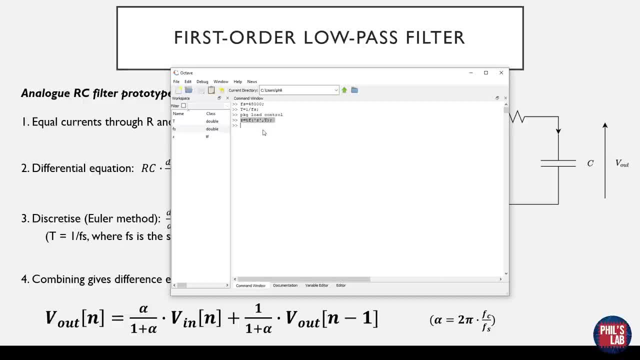 but I have a video on my channel. again, I will be leaving a link in the description which goes over the practical applications of the z transform. Using the z transform, I can convert this difference equation into a transfer function in the z domain. Before that, however, we need to define alpha, which? 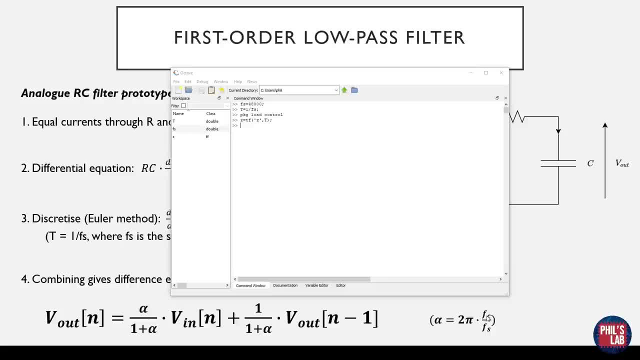 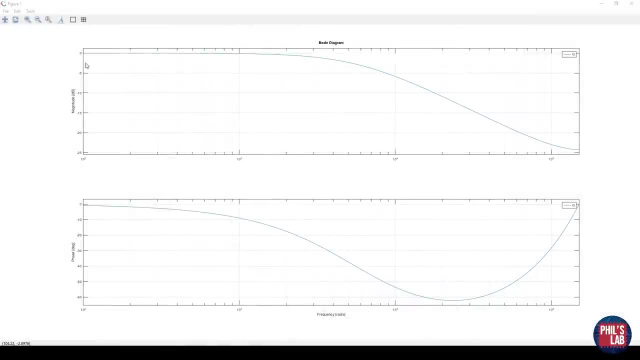 is again 2 pi times the cutoff frequency which I'll select to something like, let's say, a kilohertz divided by my sine. So once I've taken the z transform, this is my result, and then I can plot the frequency response by typing in bode of my transfer function. So you can see, here we have a low pass filter. 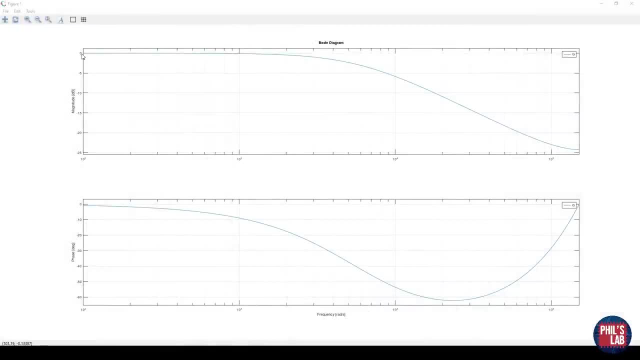 low frequencies are relatively unaffected, with a gain of 0 db, which is a linear gain of 1, and once we reach our couplet of frequency of a kilohertz, we drop down by minus 3 db to somewhere over here, and then we have a slope down and high frequencies are attenuated by about minus 20 to. 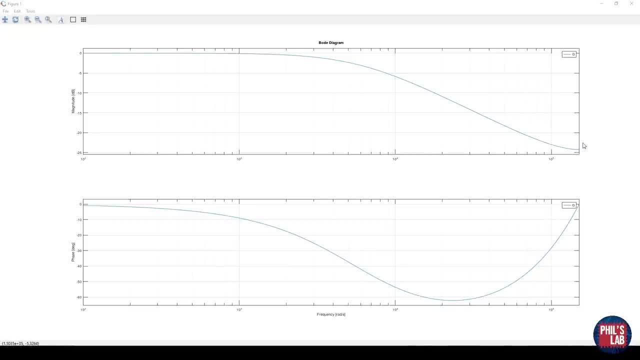 minus 25 db up to our 90.. And then we have a low pass filter which is half the sampling rate, so not the greatest low pass filter in the world. so we have pretty bad attenuation in our what is so-called a stop band and a very, very slow roll-off. The phase isn't too interesting in our case, but we can see that. 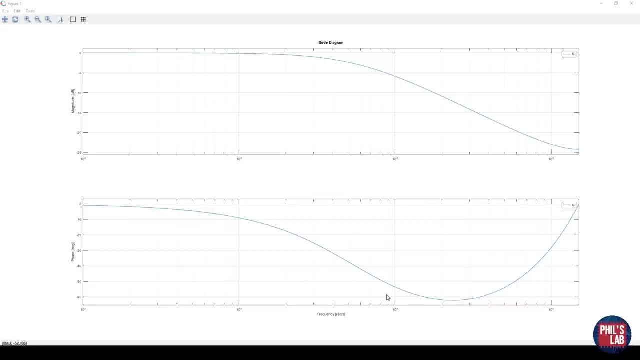 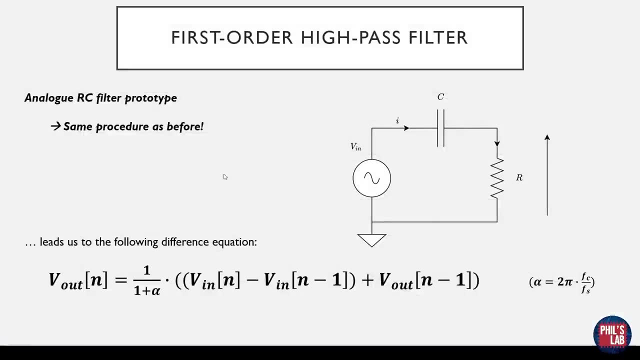 this actually adds lag into the signal later and we'll see that when we do some tests. We'd also like to look at the high pass filter, and it's exactly the same procedure as with the RC low pass filter. We have our analog RC prototype which, in this case, the R and C components are: 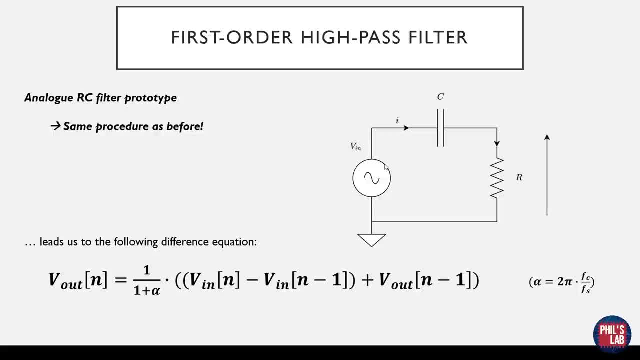 interchanged. We're taking our output voltage across the resistor and we have our input voltage feeding into the capacitor, Going through the differential equation. discretizing this leads us ultimately to the following difference equation, and that's what we're interested in. This is, then, what we can. 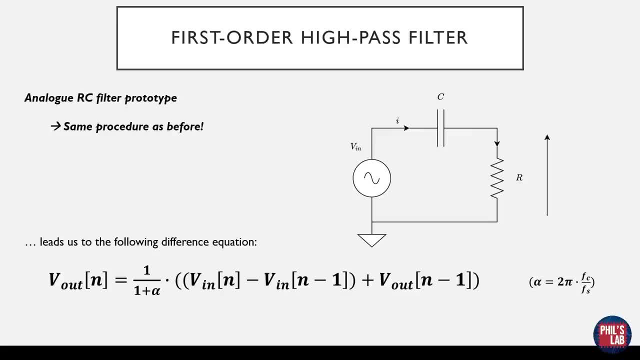 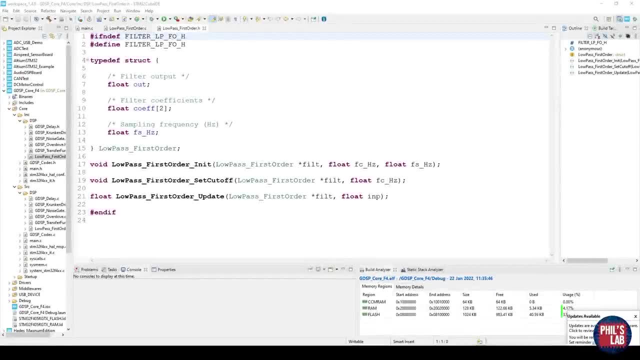 implement in software to give us our high pass filter. So now we can move over to STM32CubeIDE and implement these difference equations. So here we are back again in STM32CubeIDE and I've already written the low pass filter for us. The way I like to do it is have a header file and a corresponding 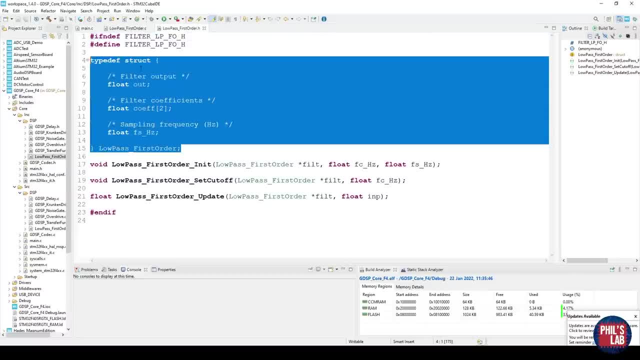 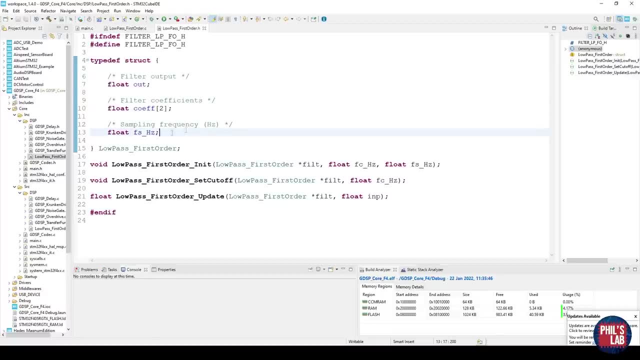 source file or c file. I'll have a struct which contains my filtered output, my filter coefficients, which I'd like to pre-compute to save us processing time when we have to do this in real time, and our sampling frequency. Then I have three functions. One is to initialize the low pass filter, so we take the. 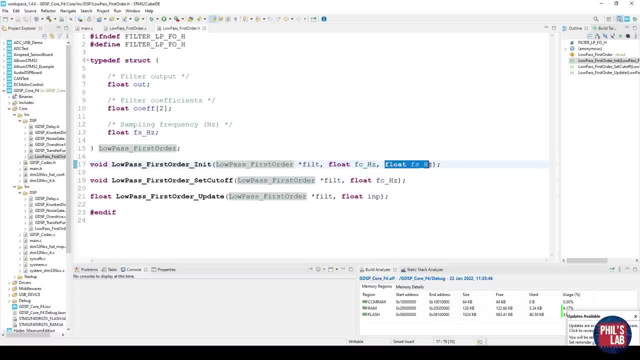 struct by reference the cutoff frequency we desire and the sampling rate of our system. Because we'd like to change filter parameters on the fly, I also have this set cutoff function which allows me to change the cutoff frequency and recompute these filter coefficients on the fly. 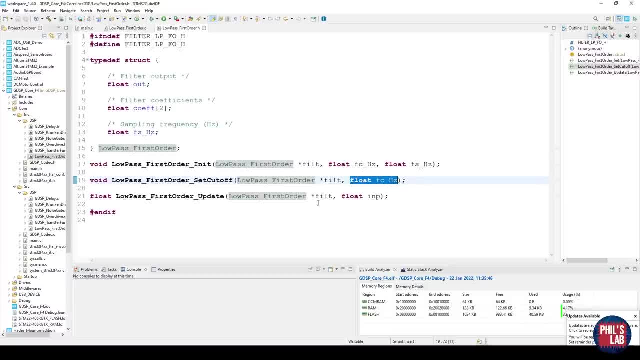 And that simply takes the new cutoff frequency as an argument and, of course, the struct. Lastly, and most interestingly, the update function is the function that gives us a new output sample when we pass it an input sample. So, going over to the c file, our initialization function simply stores the 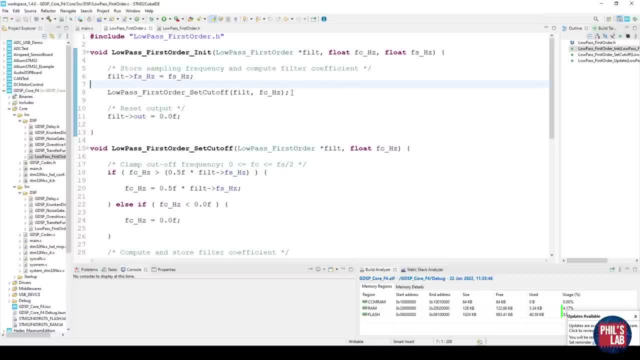 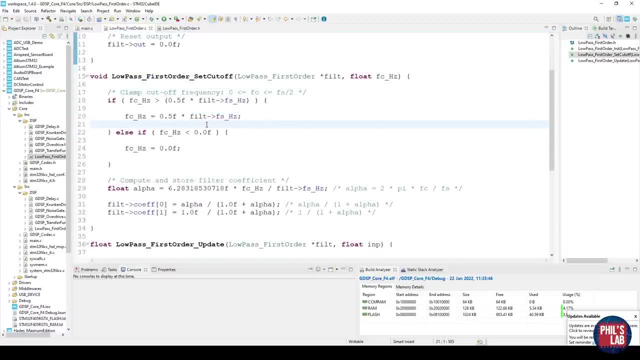 sampling frequency and then computes the filter coefficients by calling our other function, which we'll go to in a second, and also resets the filter output to be defined at zero. The set cutoff function takes of course the cutoff frequency we desire in hertz and then computes the filter. 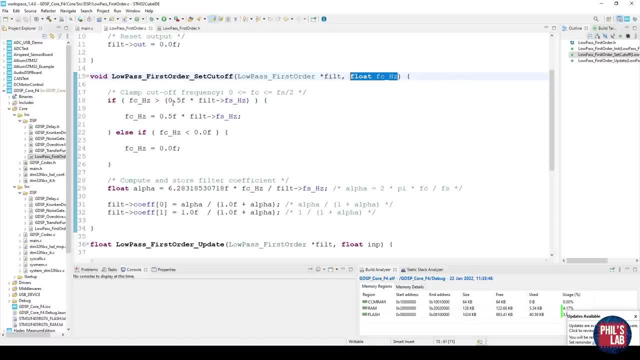 coefficients as per our difference equation. It's important to, of course, clamp the cutoff frequency, because someone might be able to type in new a cutoff frequency that is higher than Nyquist limit or negative cutoff frequency. so I'm just doing simple checks here to make sure. 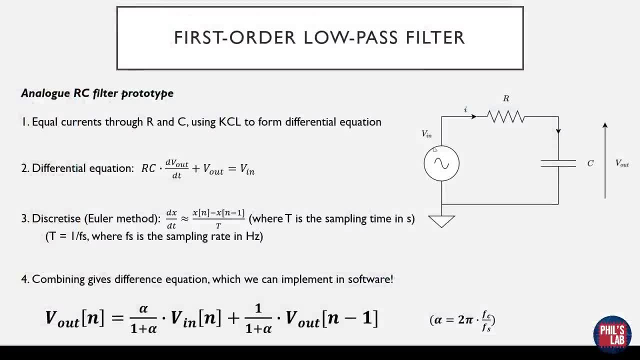 the cutoff frequency is within range. Remembering back to our first order: low pass filter. this is the difference equation we want to implement and for that, the coefficients, because we don't want to recompute these. the whole time will be alpha over one, plus alpha as our first coefficient. 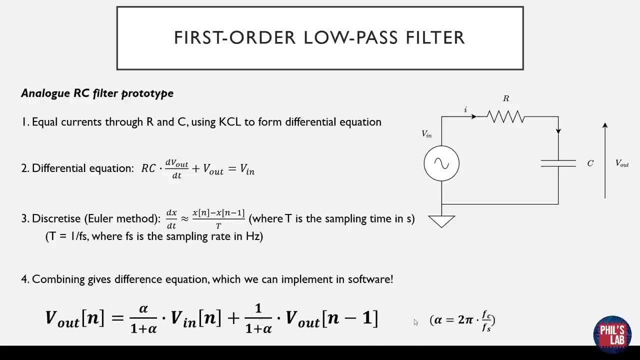 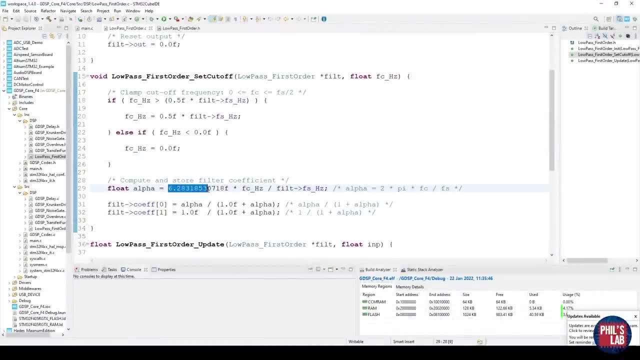 and one over one, plus alpha for our second coefficient, and of course alpha is defined as two pi fc over fs. and this is exactly what I'm doing in STM32CubeIDE. I have two pi which I have here as a constant. of course, I could make this nice as a define or something like that. 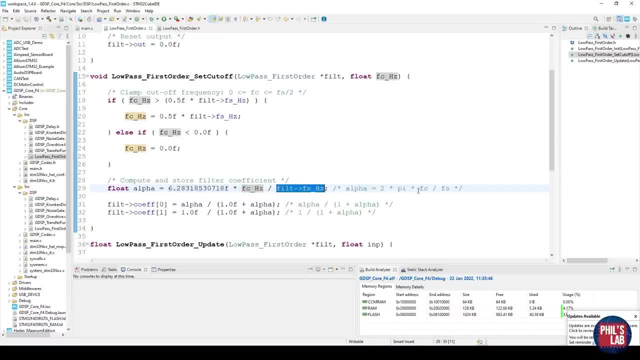 times the cutoff frequency divided by the sampling frequency. so it's two pi. fc over fs is our alpha and I can use that to compute my coefficients. Remember, the first coefficient was alpha over one plus alpha and my second coefficient was one over one plus alpha. Again, I can call this: 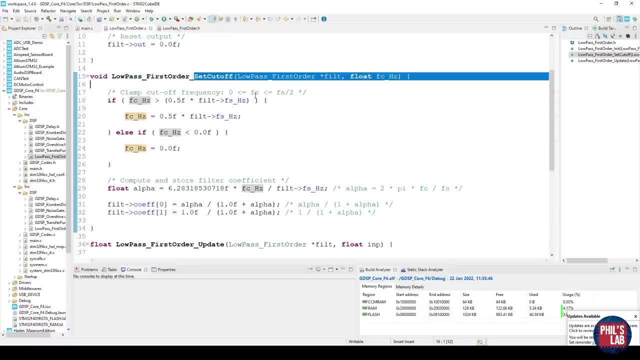 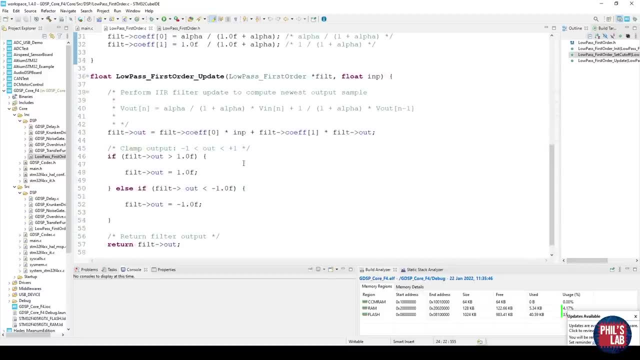 set cutoff function when I change, for example, my potentiometers on my final bullet Or my final effects pedal, to then alter my frequency response of my filter in real time. Once I've set up my cutoff frequency, of course, I can then call my update function, which actually 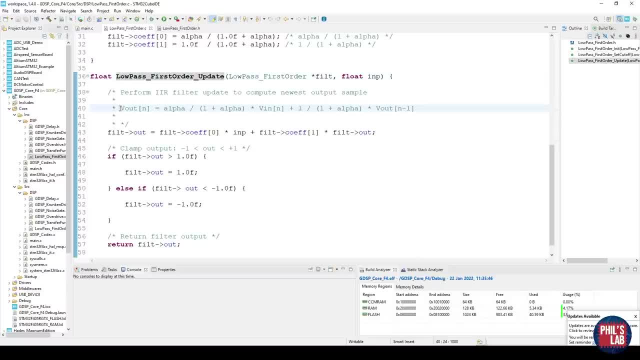 gives me the filtered output or performs this IRR filtering. We wish to perform filtering using this difference equation and again, that's all we have to implement. So our newest output is our first coefficient, which is alpha over one plus alpha times. our newest input, passed over here plus the, 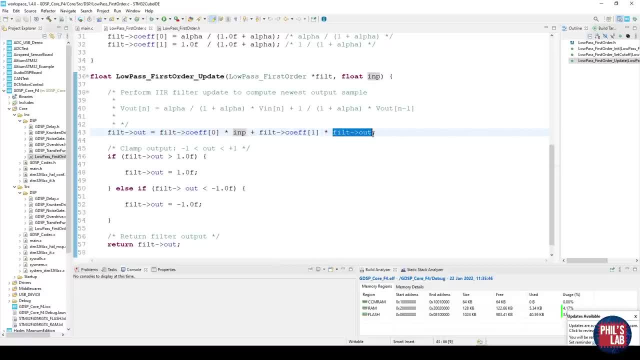 other filter, coefficient, the second filter, coefficient times my previous output and I assign this to be my new output. Then, of course, I'm clamping my output, and in this case I've made sure that my output is between minus one and plus one. So this is my clamping over here, and then I simply return my filter output. 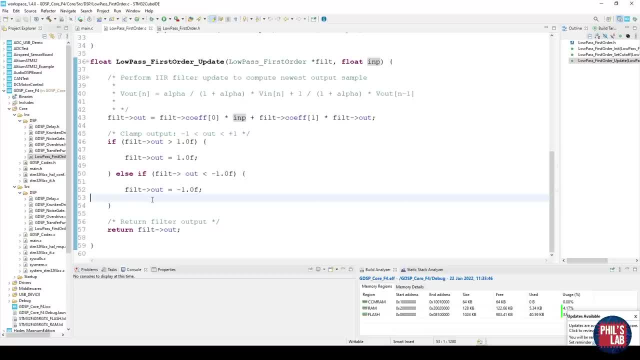 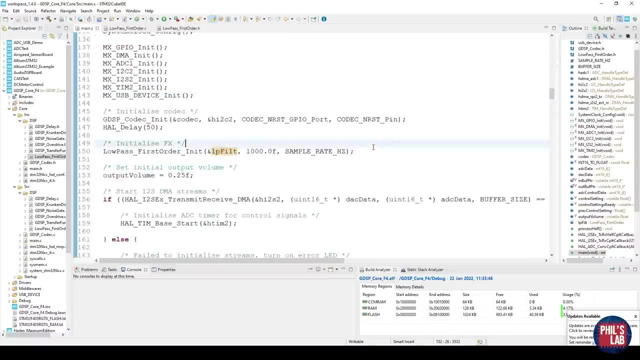 and, as you can see, it's an incredibly simple routine and this can run very easily in real time In mainc. I simply have to define my low pass filter struct, which I call lp-filt. I need to initialize my low pass filter and for now, of course, I could do this with defines again. 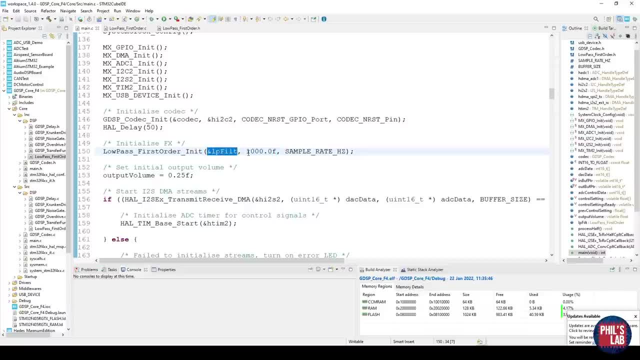 and I'm sorry for this rather crude implementation. I pass my struct by reference. I pass my initial frequency, which I'll set to one kilohertz, and my sample rate, which I've had as a define, and that's at 48 kilohertz. Then all that is left to do is, in my process, half function, which processes half of. 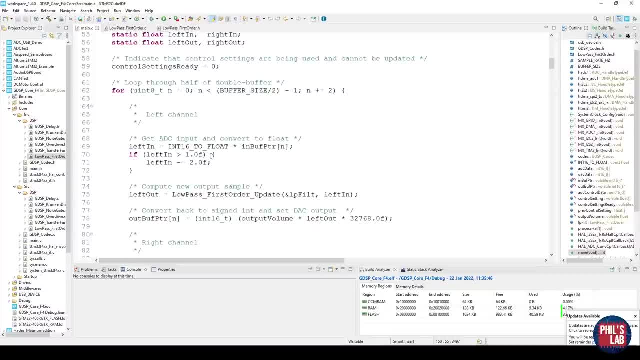 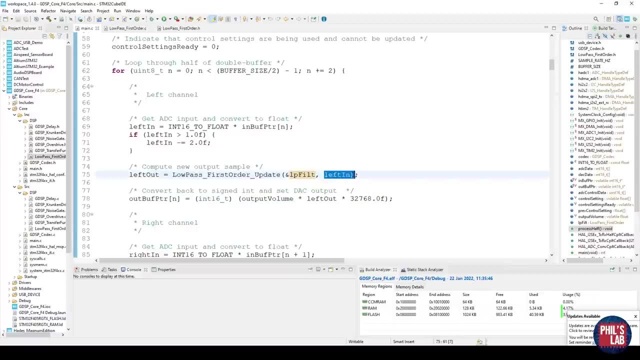 my double buffer is on the left channel, which, because we have a mono system. once I've read in my newest sample, I need to feed that into my low pass filter by passing the struct and my newest input sample. and of course this function then outputs my output sample. Then I put that: 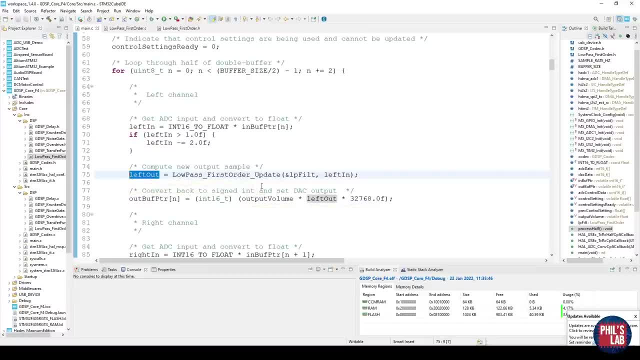 in my output buffer and send it to the codec, and that's really simple and I can flash this directly to my board. So I'll go up here, click play. I have my serial wire debug connected and this will upload the code to my STM32F4 microcontroller. There we go, download. very 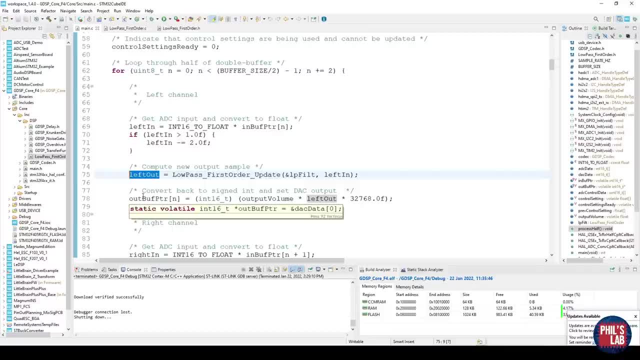 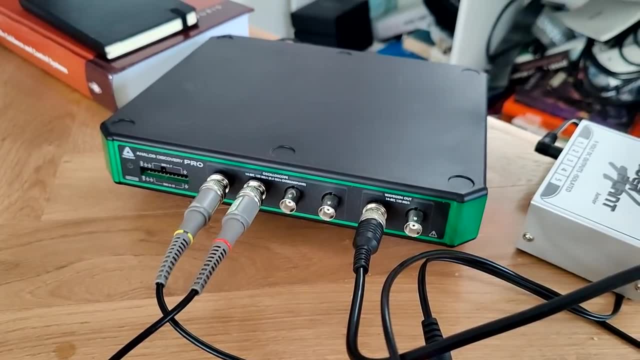 verified successfully and now let's use the Digilent Analog Discovery Pro to analyze the system before plugging this into a guitar. So this is the setup that this is running on. I have my Digilent Analog Discovery Pro. I have two oscilloscope channels, one to measure my input to 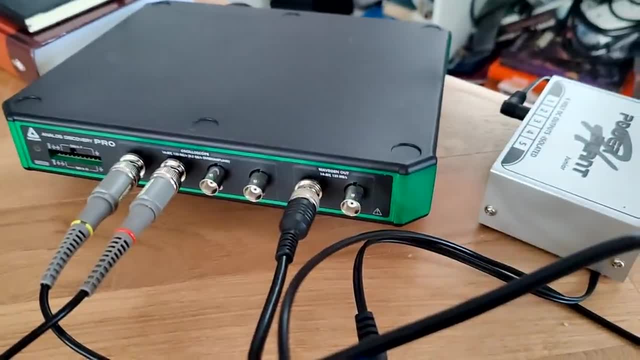 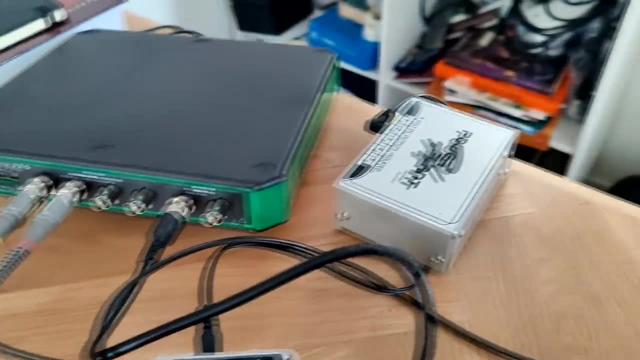 the system and one to measure the output of my system. and I have this one signal from the wave connected as a frequency or function generator to test my system and perform some analysis. I have a very simple, not the greatest power supply which provides nine volts to my input. I have everything. 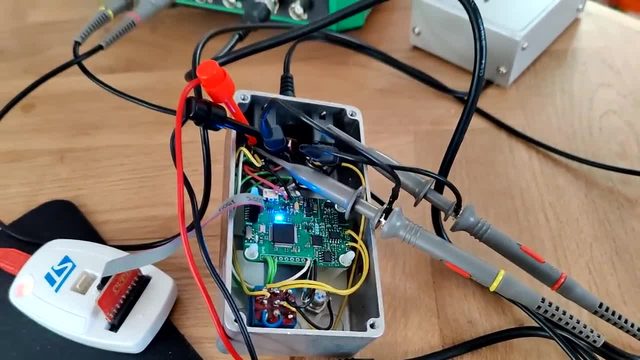 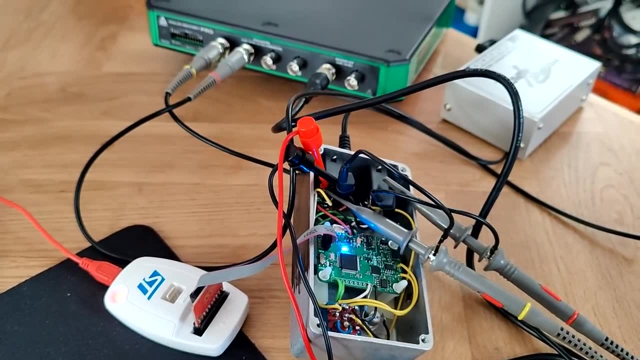 hooked up. here. you can see the board is on and running. I have all my probes connected and my serial wire debug connection as well, So let's use the waveform software to test this device and see if the filter is doing what it's supposed to. Digilent was very kind to send me one of these. 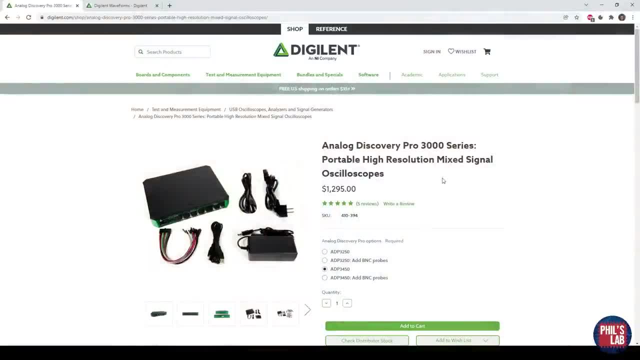 Analog Discovery Pro 3450 mixed signal oscilloscopes. and it's even more than an oscilloscope: It has four channels of oscilloscope, two channels of a function generator and various other goodies, for example logic analyzers and so on. This connects via USB or ethernet to your 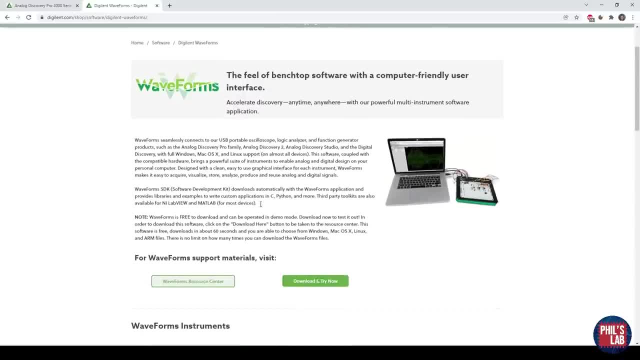 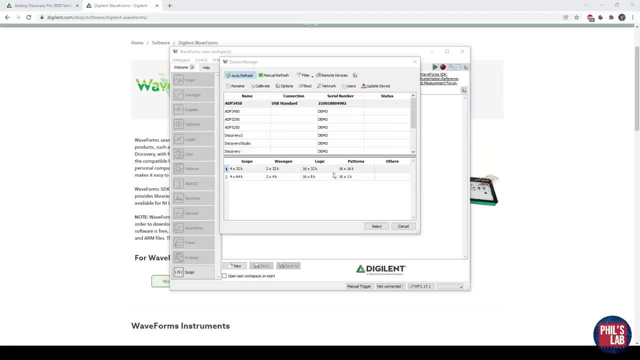 computer. This I'll be using with the Digilent waveform software, which is essentially your PC based oscilloscope. So, starting up the waveform software, it's recognized my ADP3450.. I simply click, select and then I have all of these functions over here. So, scopes, wave. 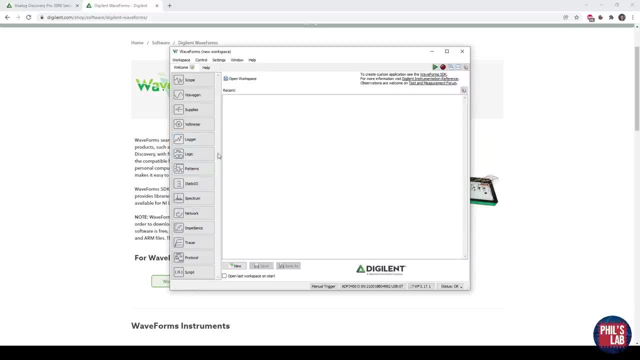 gens, voltmeters, loggers and loads of stuff which I still have to explore. What we'll be using is the scope and the wave generator to do, for example, time domain analysis, and we're using the network analyzer to give us a frequency response plot. Lastly, on the note of making 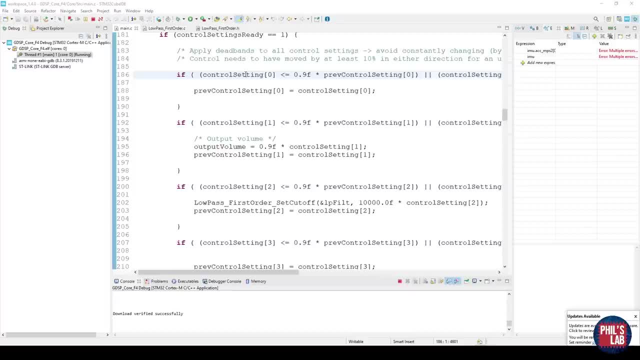 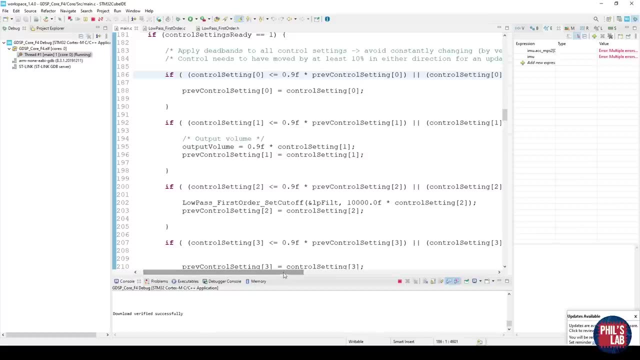 this filter variable, I'm reading my control settings. so once I have a flyer from my ADC that is the control settings ADC, I'm reading the control settings in applying a small dead band and if the control setting has changed by more than 10 percent, I'm readjusting. 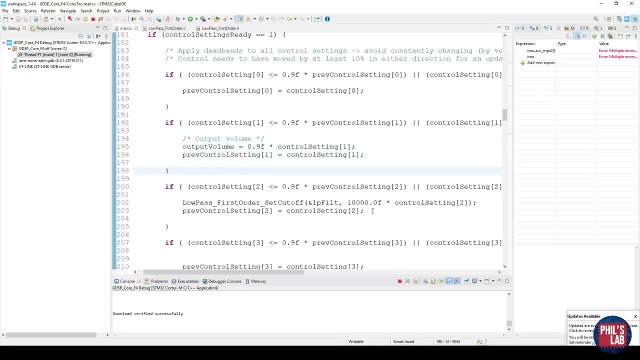 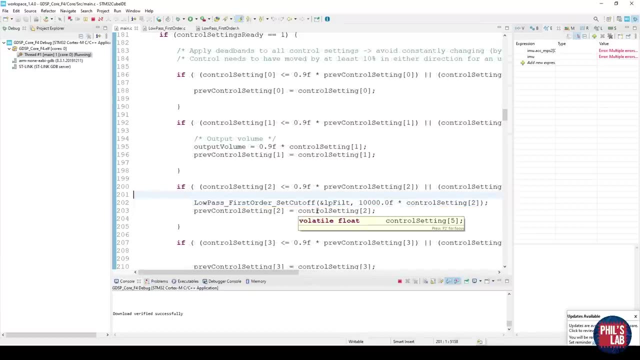 In some sort of parameters, and this is one for the output volume and one for the control setting for the cutoff frequency of the low pass filter. We also have a third pot enchantment available and we'll be using that for the high pass filter cutoff, which we'll see after we've analyzed the. 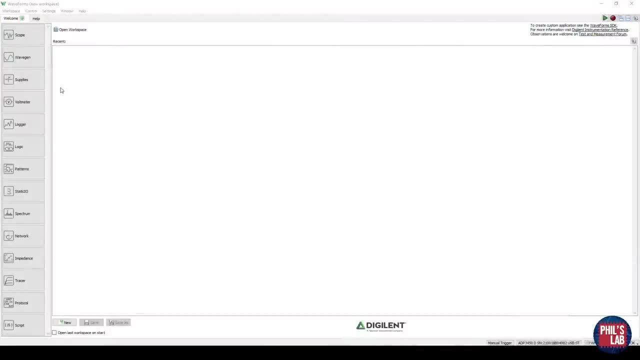 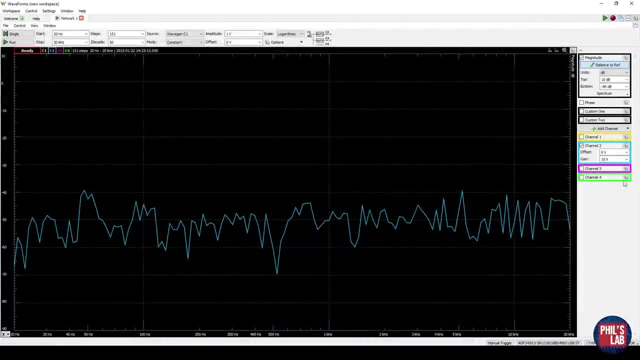 low pass filter. So here now in the software, I would like to use the network analyzer first, which I can use to give me some sort of frequency response analysis. So I click on that on the right here I can choose which channel to analyze, and I'm on channel 2 which is my output of the effects. 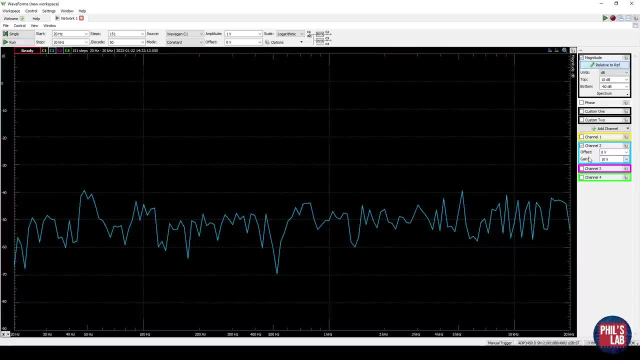 pedal. I am using a 10 times per second frequency response, So I can choose which channel to analyze, and I'm on channel 2, which is my output of the effects pedal. I am using a 10 times per second frequency response, So I need to set my gain to 10.. My source is the wavegen channel 1. 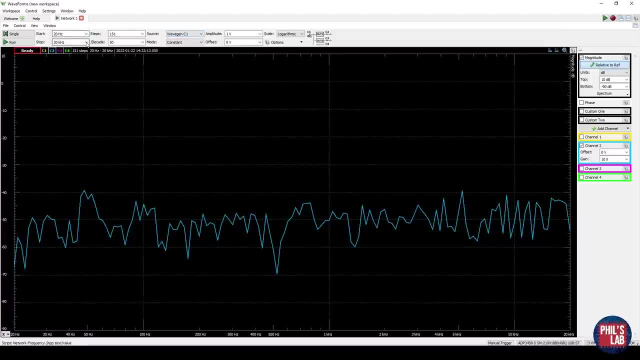 and I would like to- because we're in the audio range- go from 20 hertz to 20 kilohertz. Of course you can go a bit lower, a bit higher, just to see the full frequency response. but now I have my potentiometer for my control set to right in the center, So if I click on run I can start an. 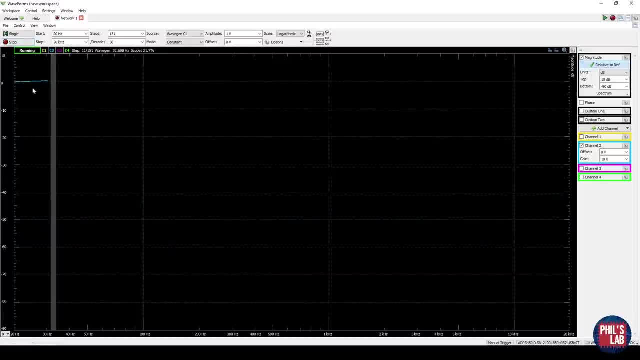 analysis and you can see, at low frequencies, because we have a low pass filter, the signal is relatively unaffected. we're at about zero db. Now I haven't quite centered my volume control, so it might be a bit around zero db. and now the analysis is complete- at least one of them I've 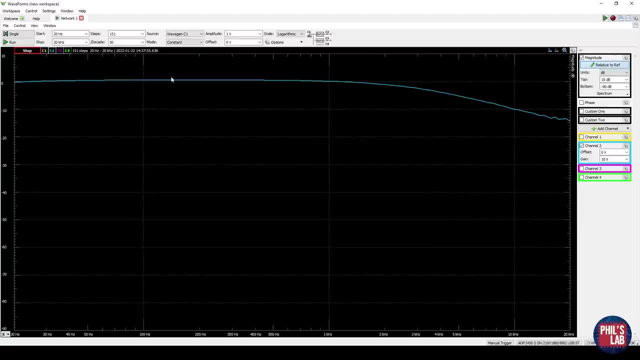 clicked on stop and you can see we have our pass band here, which is relatively flat, and then we have a slow roll off as we saw in octave or matlab. Now keep in mind this is not with a one kilohertz cutoff frequency. I've played around a bit with my cutoff frequency control using the potentiometer. 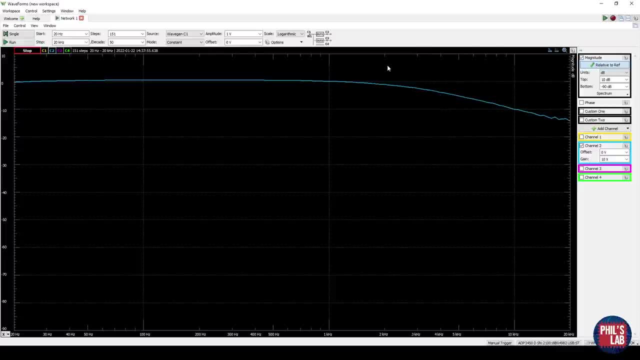 so we can vary this. so if I change the cutoff frequency now just using the potentiometer and then re-click to do a single measurement- so I've moved my cutoff frequency quite a bit lower- now I can use this measurement tool to find the minus 3 db point. now, keep in mind, up here I'm at about 0.4 db, so it's minus 3 db down from that. 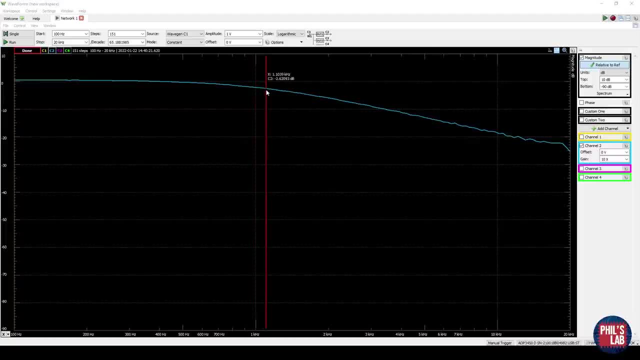 it's about minus 2.6 db and that's about 1.1 kilohertz. now let me just readjust my potentiometer and do another measurement. and now I've adjusted my potentiometer, done another reading and again I can find my minus 3 db point. so it's about 800 hertz, and of course I can turn that the other way. 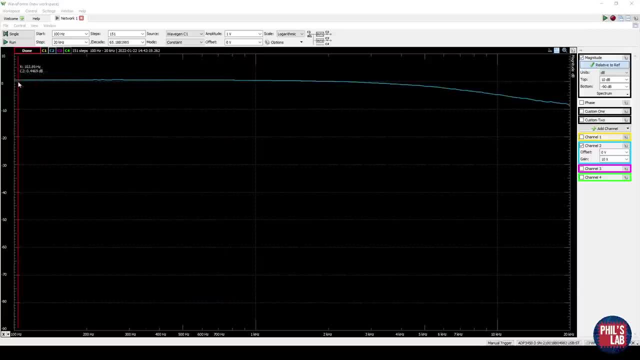 as well. and here you can see the cutoff frequency is quite a bit lower. so I've moved, my cutoff frequency has moved. so again minus 3 db from here, so minus 2.6 somewhere over here, and it's moved to 6.3 kilohertz. so we've verified, we actually have a low pass filter, but we've also 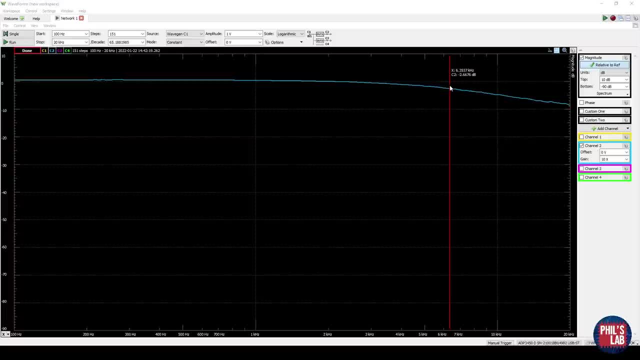 verified that we have a variable low pass filter so we can change the cutoff frequency simply by changing the potentiometer. one thing we also need to verify is if the volume control works. so now we have the volume control centered at about zero db and I see if we can get a. 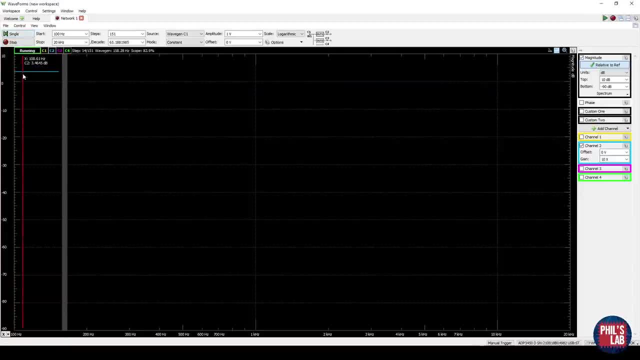 bit of boost out of it. click rerun and you can see we've got a boost of about three db now and of course we can do also attenuation with our volume control and we have a cut of about minus 11 db. so that seems like it's working. we have a variable low pass filter, even though not 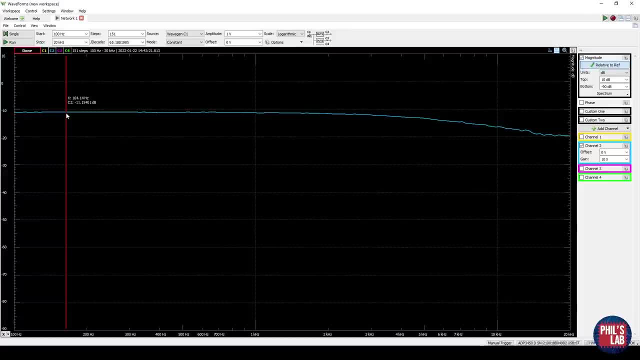 a great one. it's a simple first order low pass filter. we've done a pretty bad approximation with the Euler method and we have a working volume control. now we can implement the high pass filter in cascade with this low pass filter, essentially forming a very simple bandpass filter. 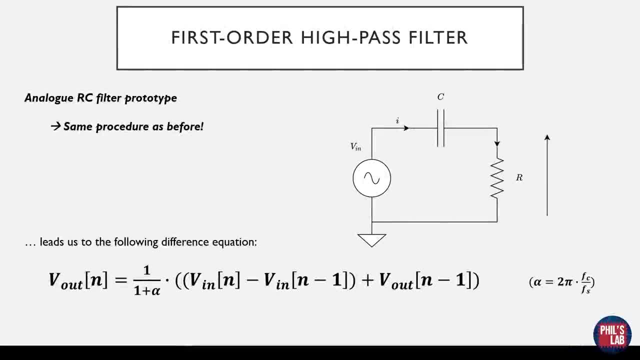 so now we can try- after we've analyzed this low pass filter at least a tiny bit, we can move over to the first order, high pass filter, and it's exactly the same procedure, except that we're now implementing this difference equation. the way I've done that in stm32q by de is then simply: 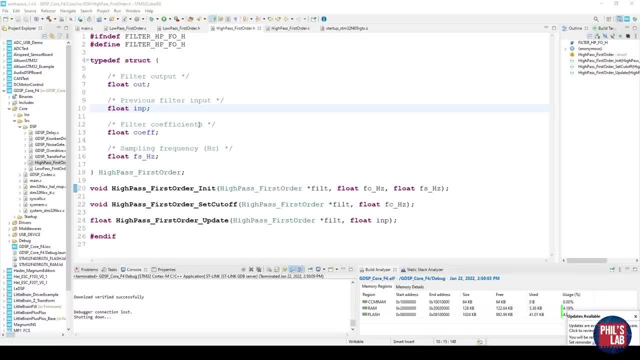 take my low pass filter, header and source files and change them a tiny bit. the high pass filter: because of the difference equation we also need to store the previous filter input, so I've added that to the struct. but other than that the header file is identical. going to the dot c file, we also 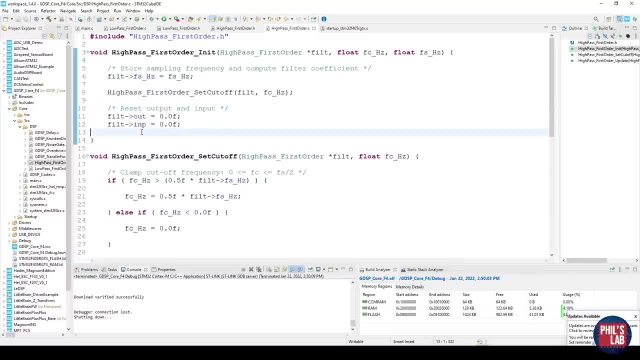 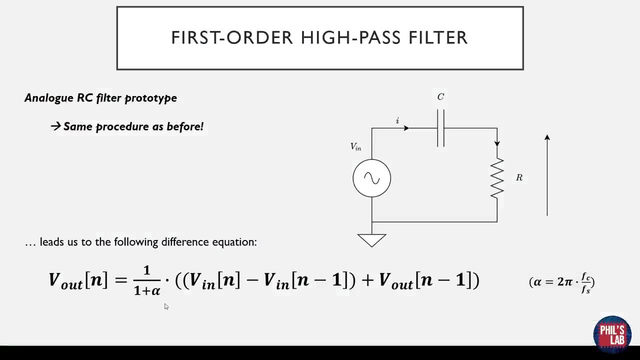 have to reset the current output and the previous input. so I've added that here and we have to change the filter coefficient calculations. we only have one filter coefficient and this is one over one plus alpha. then we have this difference between the current and the previous input sample and 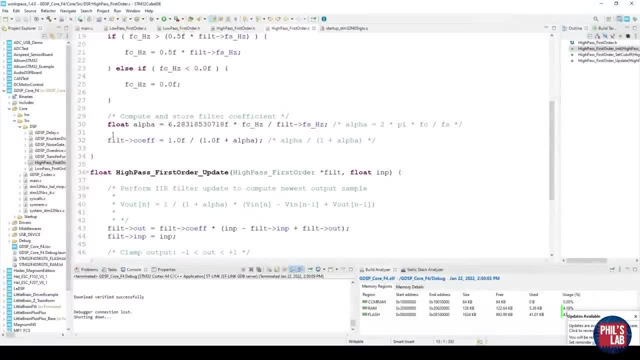 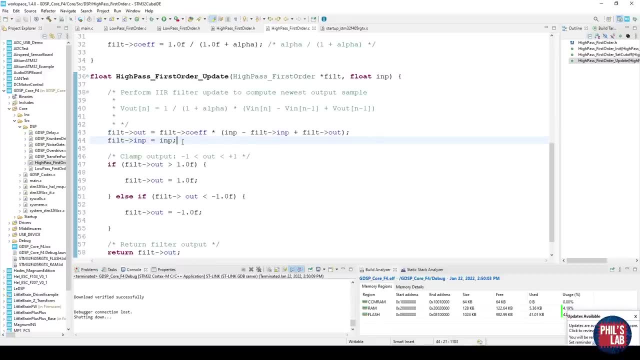 we're adding the previous output sample to form our output compute and store my filter coefficient, and then I compute my output here in the update function simply using the difference equation and then storing my previous input same as before. so I've uploaded that code already to my board. 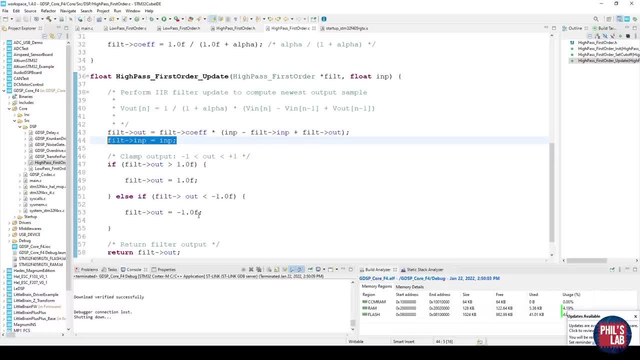 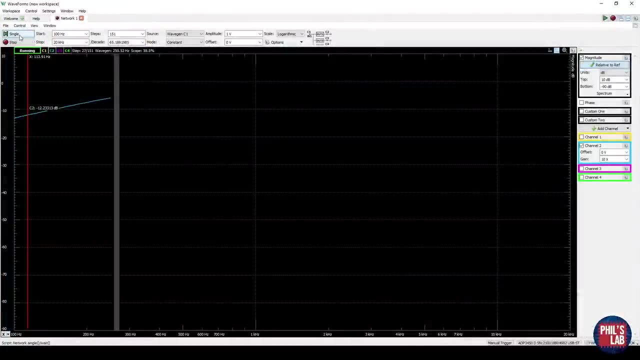 and we can go back to waveforms with the digital and analog discovery pro to test it out. with the controls pretty much centered I can run a single measurement. so I have my low pass filter and my high pass filter engaged and try to match my mid band gain to about zero db and you can see. 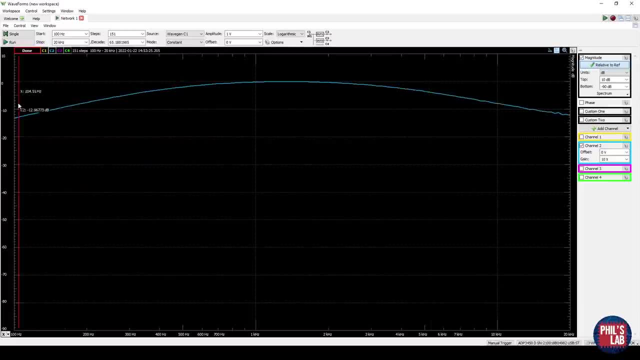 over here, since we've added the high pass filter. now low frequencies are affected by the high pass filter, which only allow high frequencies, and up here we have the low pass filter, which affects high frequencies so effectively. we have a bandpass filter by cascading a low and a high pass filter. 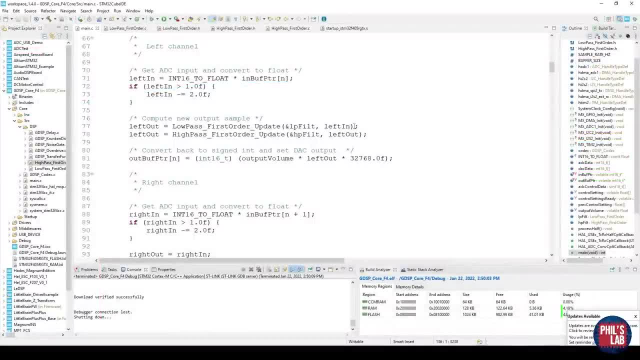 the way I've actually cascaded these filters is I take my input sample, which is my raw data passes through my low pass filter and then pass that filter data through my next filter. now, keep in mind the order really doesn't matter for these linear filters. I could do my high pass first and then my low pass. either way doesn't really matter. 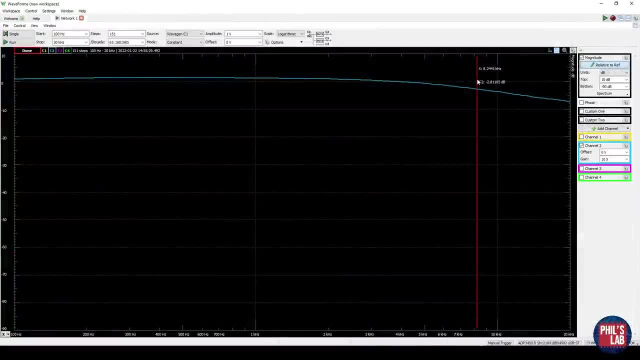 so it looks like we have variability in our low pass and high pass filters. they're both working essentially the same time by feeding into one another, and we have volume control. I'd also just quickly like to look at the time domain behavior, so to see- we have to see- any. 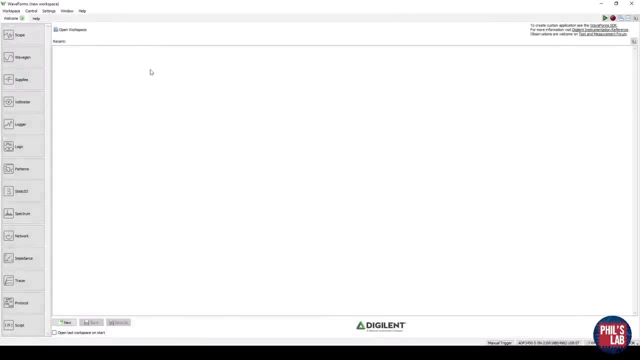 phase lag, if we can match amplitudes and so on. the way to do that with this, waveforms and the Discovery Pro- is to go back to the main workspace, and we are going to use the scope and the wavegen. So the wavegen lets me generate arbitrary signals. in this case, I just simply want a sinusoid. 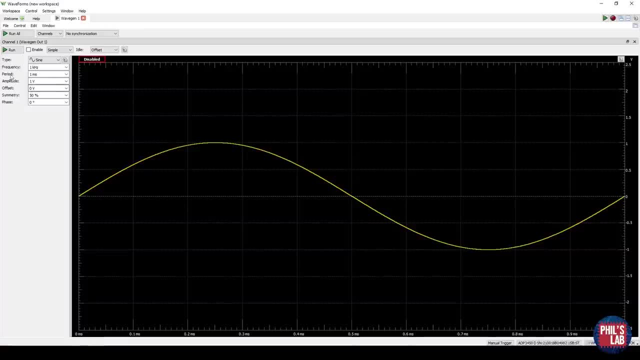 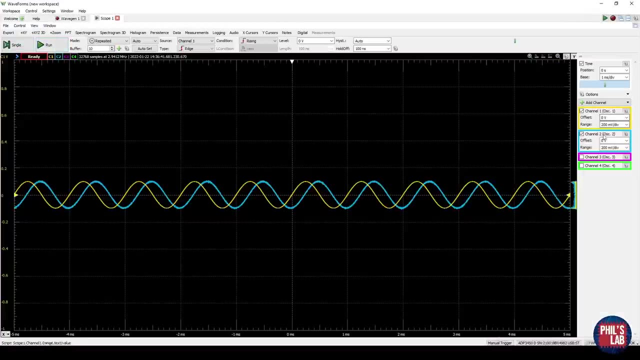 let's just say one kilohertz of an amplitude of one volt, no offset, and click run. and then I need to go back and look at my scope over here and then I need to click run on that. channel one is my input, channel two is my output. so if I go here, if I play with my volume control, you can see it's. 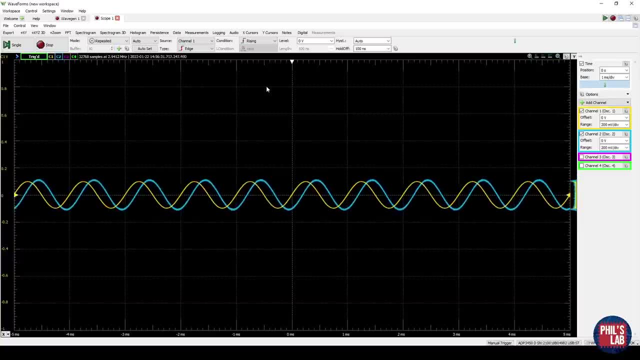 going in steps. I can change my volume, like so, and of course I can change my cutoffs. so if I change my low pass filter, so you can see, I'm decreasing the cutoff ring to my low pass filter and that's giving me more attenuation at this one kilohertz. or of course I can move it back again and you can. 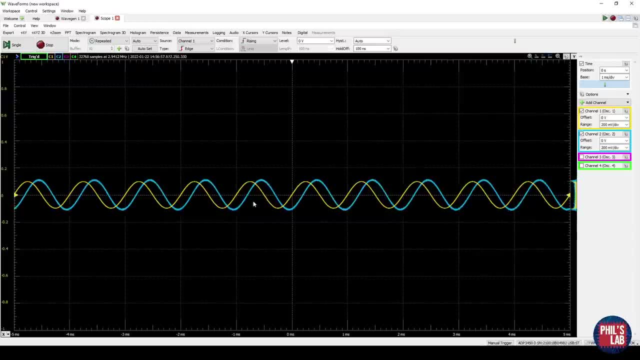 see I'm getting less attenuation. you can see also my yellow trace is my input, my blue trace is my output and you already see this phase lag or this delay. this, of course, is what we expect when we filter a signal. we haven't looked at the phase response in detail, but we will have some sort of 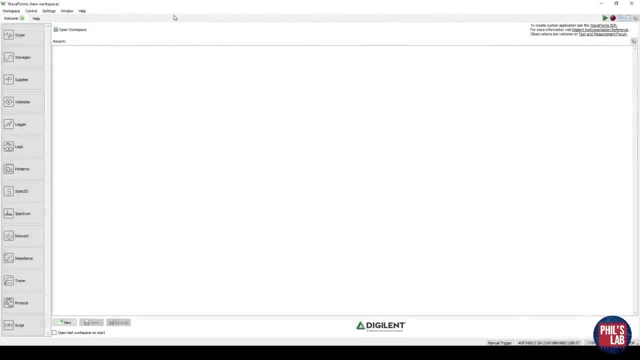 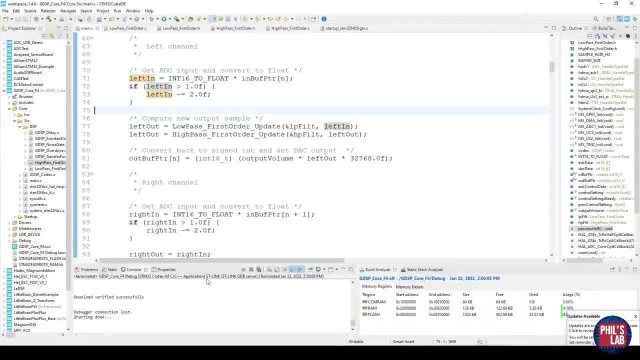 phase shift, Especially if you move high end frequency. so there's many more things I need to explore with this waveform software, as well as with the Analog Discovery Pro, and I'm sure I'll feature this in many videos. so far, it looks like our high pass and low pass filters are working, so let's move over.